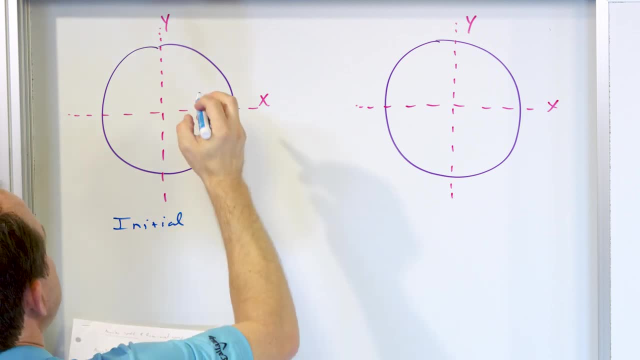 I'll call this initial Initial. So what we have is from the center of the circle, as measured, to the edge of the circle at some radius r, and it makes some angle. I'll call it theta sub one with the x axis. all I'm doing is saying this ray, we have to measure its position somehow. we're calling. 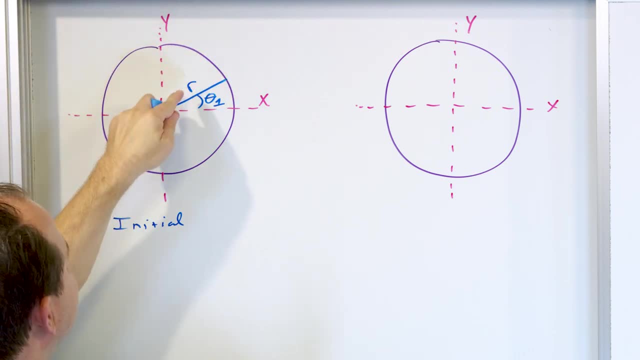 this r, which is just means a radius of the circle right. And as we sweep around, the radius of the circle stays the same. So how do we measure its position? we measure it as an angle to the positive x axis. So the initial position of this ray in this position is measured theta one. theta sub one. 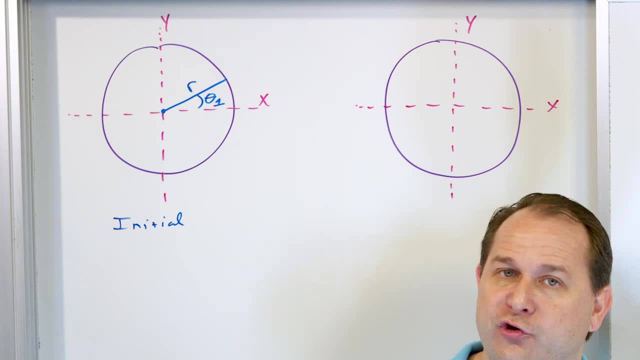 radians from the x axis could be 10 degrees, if you're working in degrees, or could be more appropriately expressed in radians: some radian measure from the x axis. Now what's going to happen is we're going to allow some time to elapse. 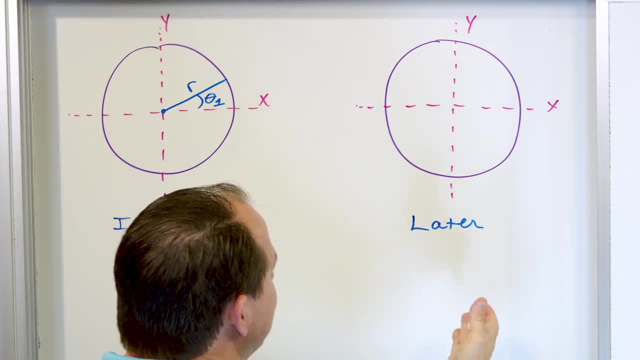 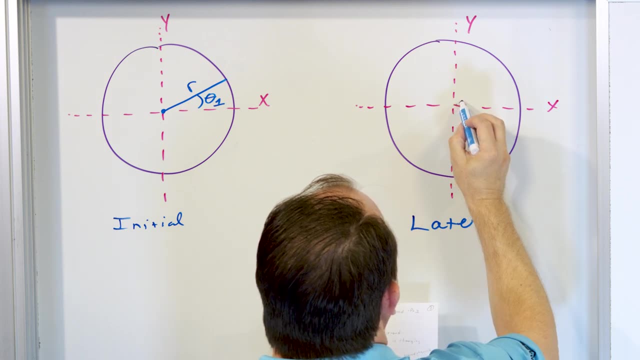 All right, And so we're going to say later, how much later? Well, it depends on how fast this thing is rotating. we're going to consider it to be like five seconds later or whatever. So initially you can the initial position I'll draw there and kind of superimpose on there. But really I'm mostly 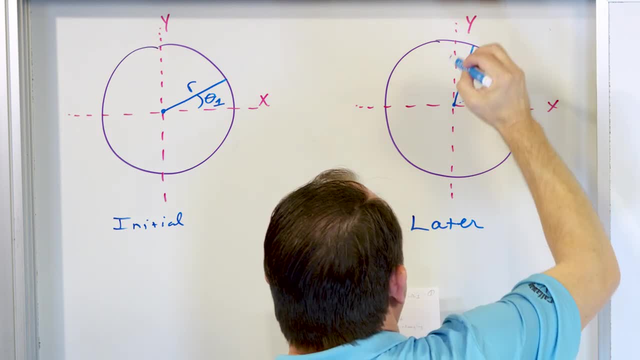 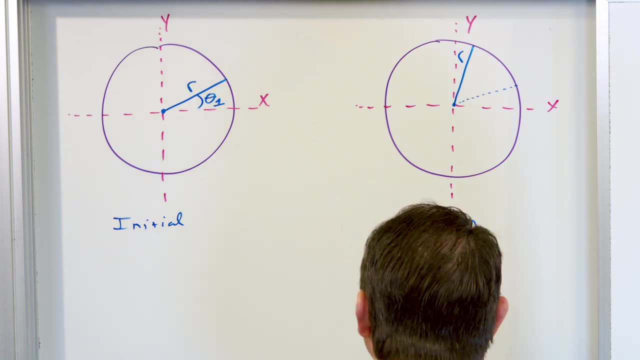 interested in drawing the final position of this thing, which will be like up here right Now. again, it has some radius r and the position of this ray is always measured with respect to the positive x axis, So really it's measured down here. 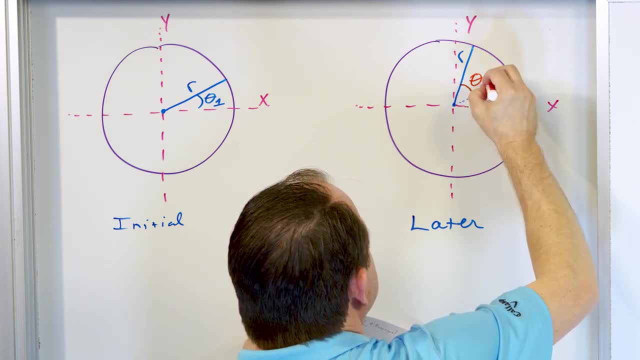 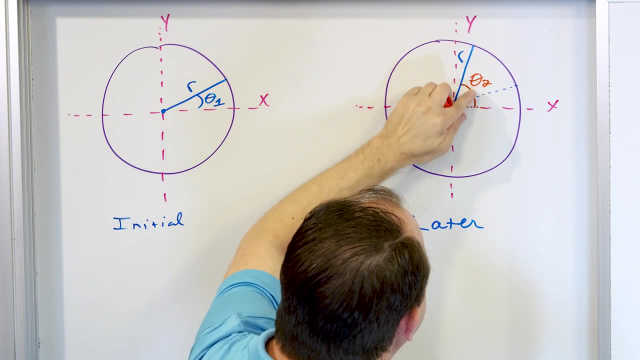 Like this. we'll call it theta sub two. So this dotted blue line is just there for reference. okay, it doesn't have anything to do really with the final position which is here. it has some new angle again, measured with respect to the x axis. So you can see that initially had a small angle. 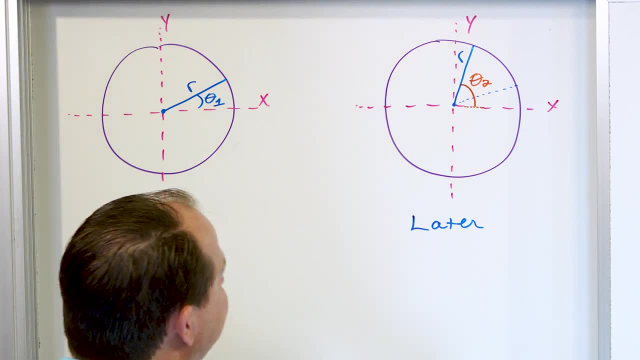 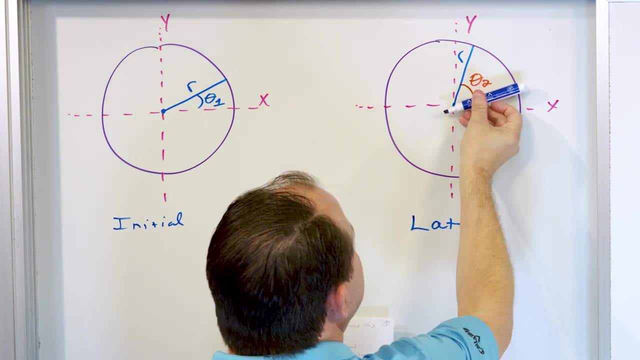 some seconds later it has a larger angle. we just call it theta sub two. Now, as this thing rotates from here to here, initially it was in this position and then it moved to this position. So, as it rotates from the initial to the final position, it's going to be a little bit smaller. 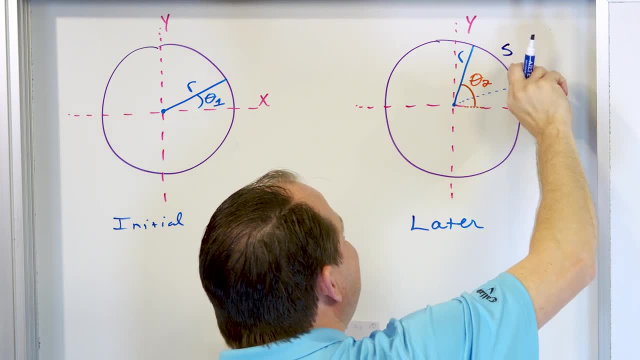 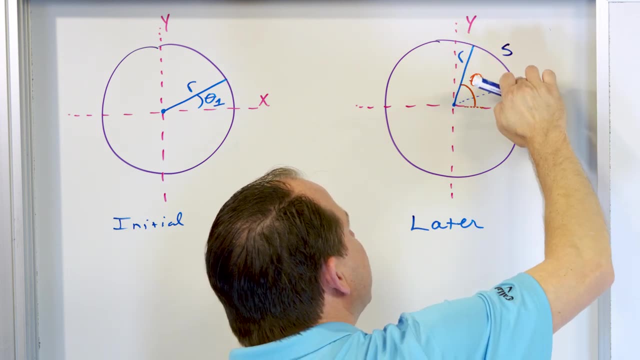 to the final position we say it goes. the end of the thing sweeps out in some arc length from here to here, because initially it was here and then it goes here, And so if you could add up all the distances the tip of the thing traveled, it would be some arc length, which we've already. 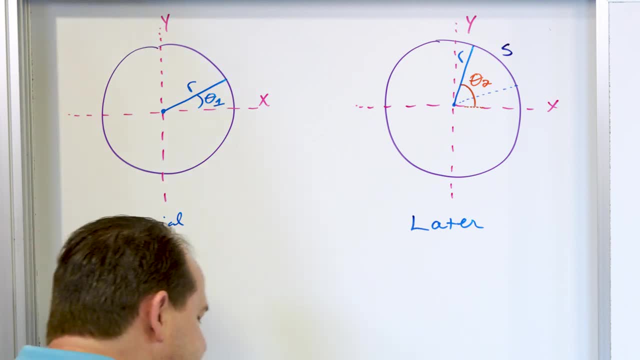 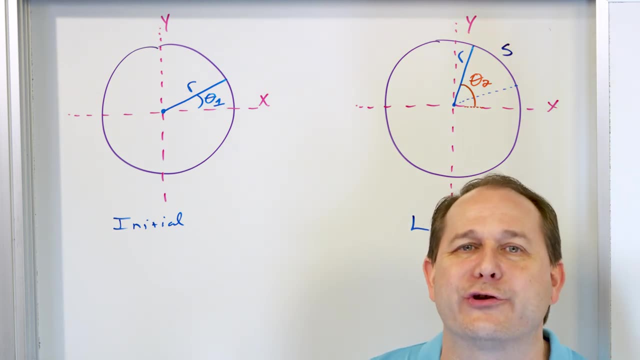 talked about arc length in the last lesson, So if we wanted to figure out, remember where we're going with this- is trying to figure out how fast things rotate in terms of the angle, the angular speed. So I'm not talking about meters per second, That's just a straight line speed, I'm talking. 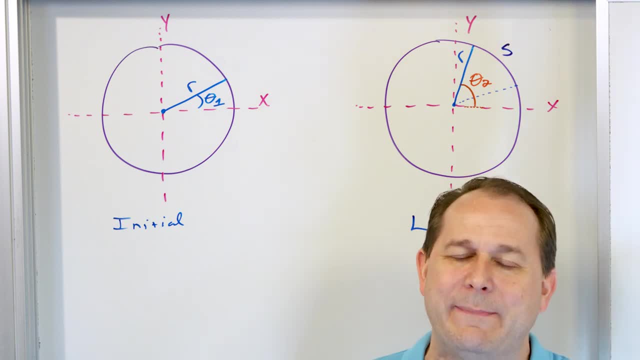 about angular speed. How many radians does this thing sweep out per second? If it's a very high number of radians per second, let's say it's like two pi radians per second. Remember two pi is all the way around the circle, So two pi radians per second would mean all the way around the circle. 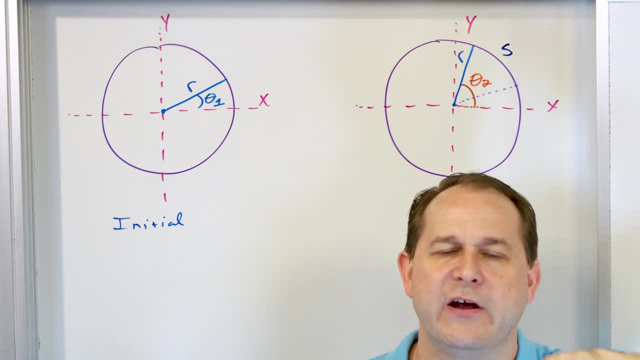 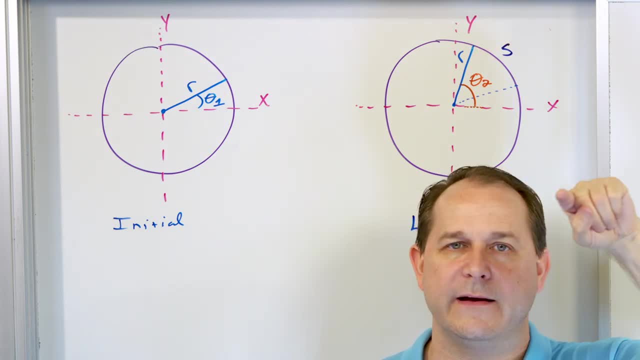 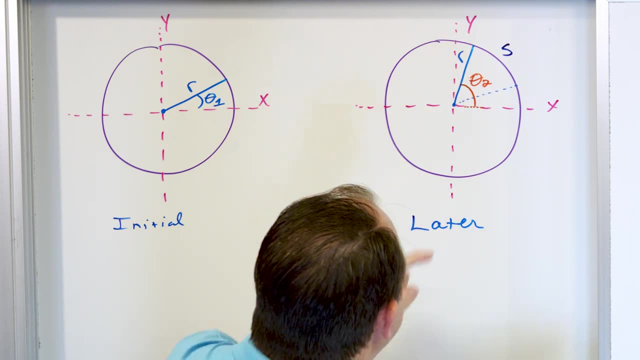 half of that original rate. Well then it's going to be sweeping out half of the angular speed where the angle is what you're measuring here. So if we started angle theta one and we end up at theta angle two, what is the difference in the angle? We can call it a delta angle- the difference in 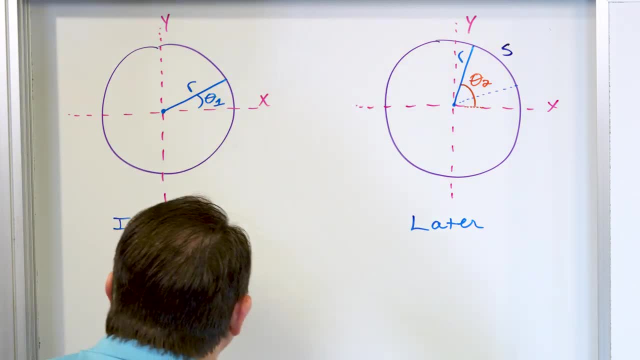 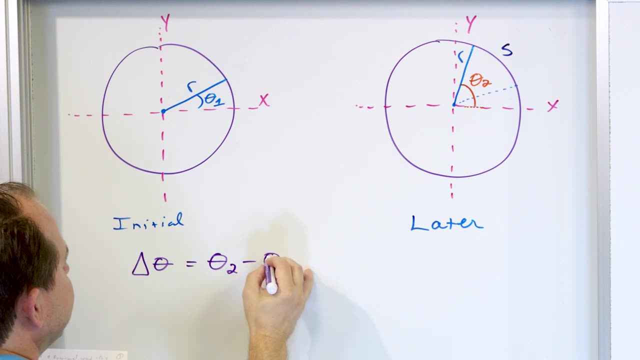 the angle between state one and state two. So what we can do is we can write down, is we can say that delta theta, which is just the difference in the angle between state one and state two, is theta two minus theta one. So if we start out, you know, at some small angle and end up at some 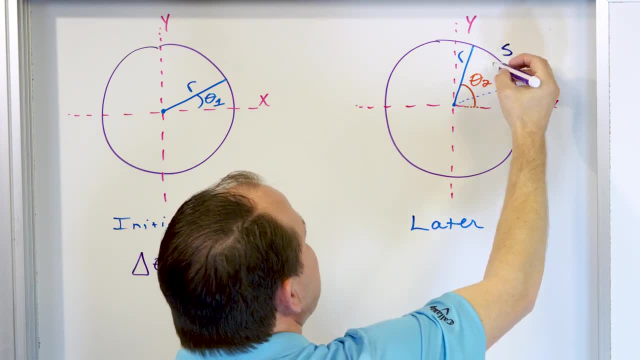 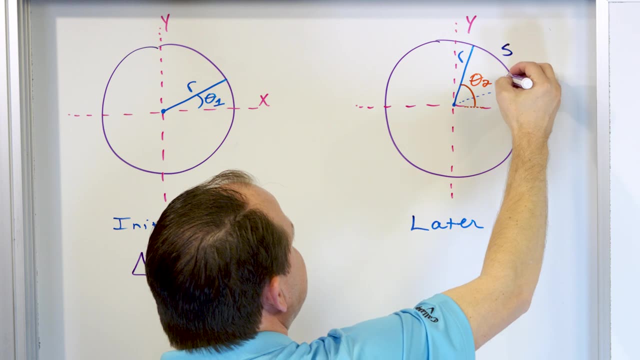 larger angle. we subtract the angles and that's going to measure. that's going to measure the difference in the angle from the starting position here, at the dotted line, to the final position here. When we subtract these two things, we're going to get the delta angle. that is swept out. 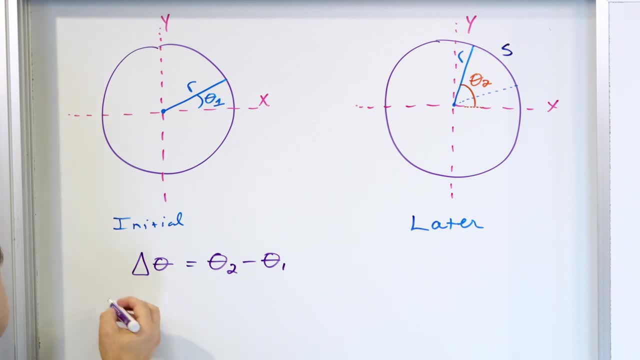 from the starting position to the final position. All right, And that's what it is. It's just a subtraction. So let's just say that this sweeping out of this angle takes whoops. if I can spell take correctly, takes t seconds. So let's say that we sweep out from. 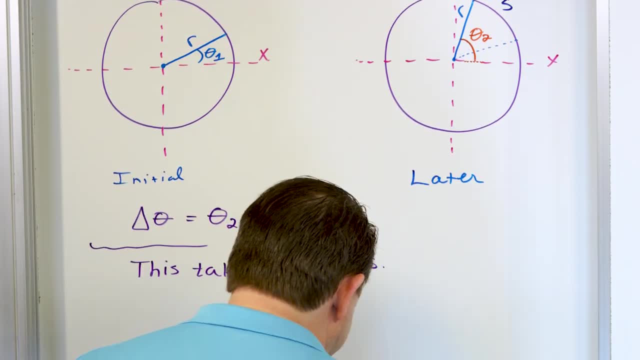 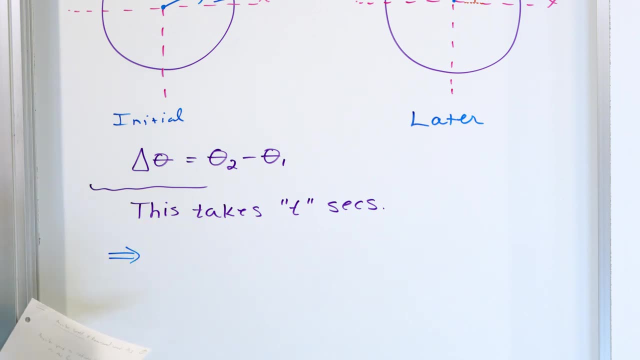 position one to position two in however many seconds it takes. we call it t seconds. Then what we can say is that we can define what we call an angular speed, angular speed, And we call angular speed lowercase Greek omega, which is like a W, but it's like a curly W, right, I know. 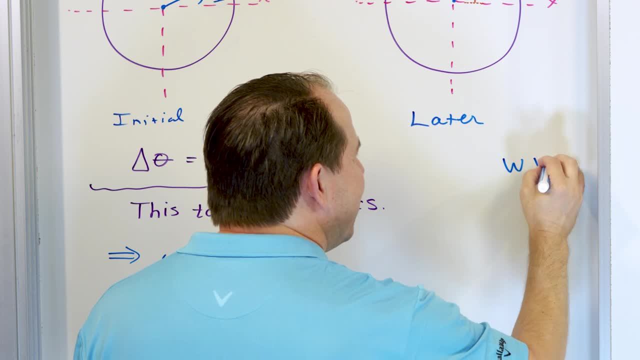 that it looks a little weird, but a regular speed is a regular speed. So if we subtract the angle that's taken from the starting position to the final position, we get a regular W. A regular W is like this. That is not omega. Omega, lowercase omega is a curly W, like this Capital omega. you've 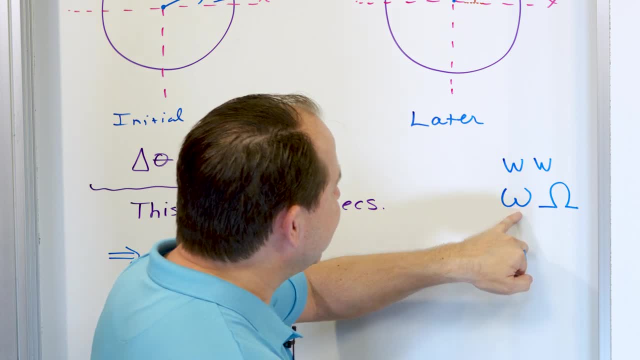 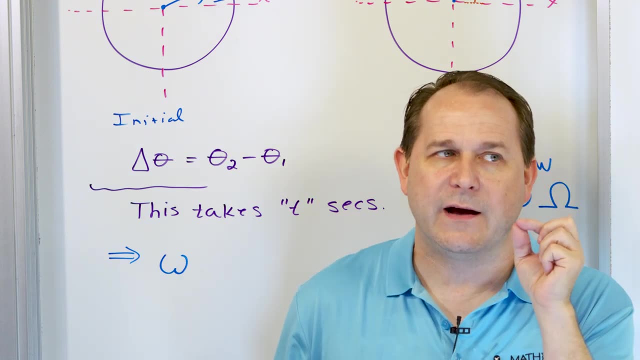 probably seen is this: This is a capital Greek letter. omega. This is a lowercase Greek omega. We use omega, lowercase omega, almost all the time for angular frequency. It is a Greek letter that you will use forever in physics, electrical engineering, mechanical engineering, aerospace. 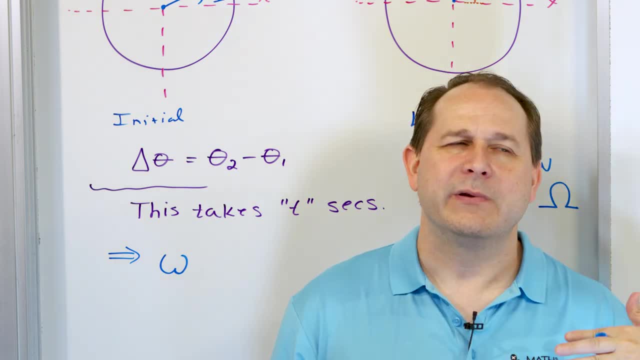 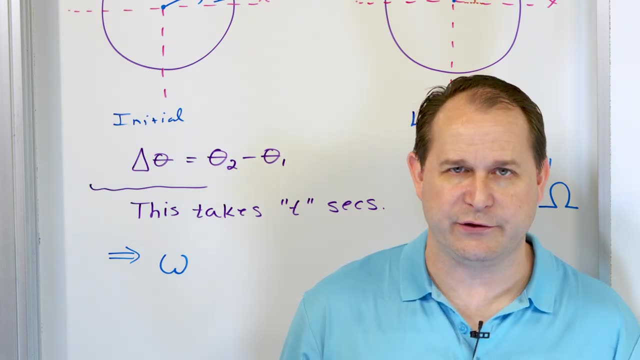 engineering, mathematics. You don't use it so much in chemistry because we don't talk about angles, although we do, for angular bonds, angles between bonds in chemical molecules, right Or in molecules. But this is the way you want to draw it. 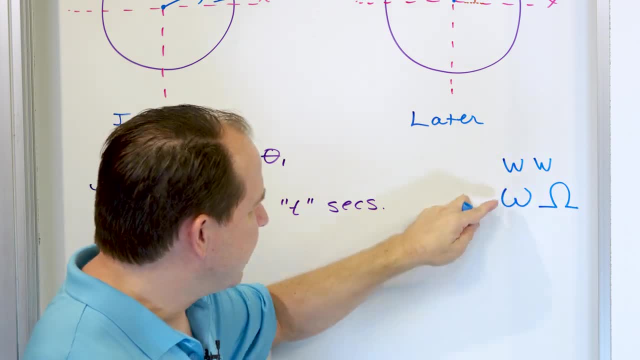 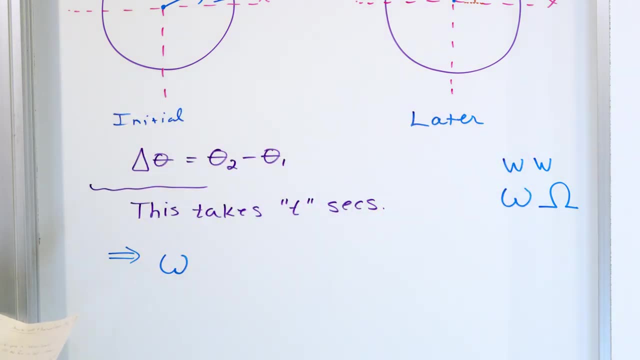 You want to draw it with a nice kind of a rounded bottom. essentially, I'm trying to say it nicely, but a rounded bottom, That's the way you want to draw it. That is lowercase omega, And what it is is the angle that you swept through from the initial to the final state. 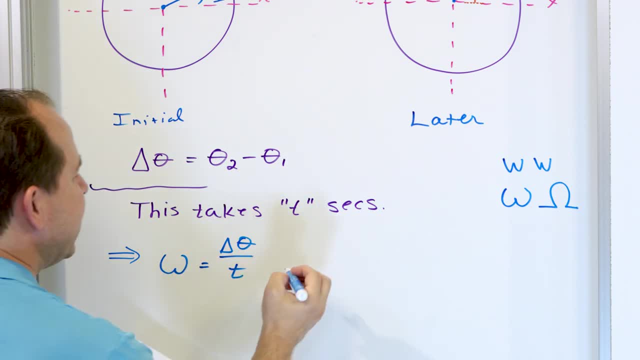 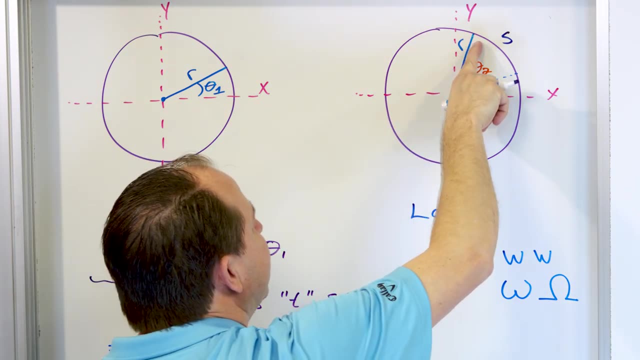 and you divide it by however many seconds that took, And what you get for a unit is radians per second. Because on the top, when you subtract the angles, what you're doing when you say theta 2 minus theta 1, you're figuring out how many radians did you rotate through? 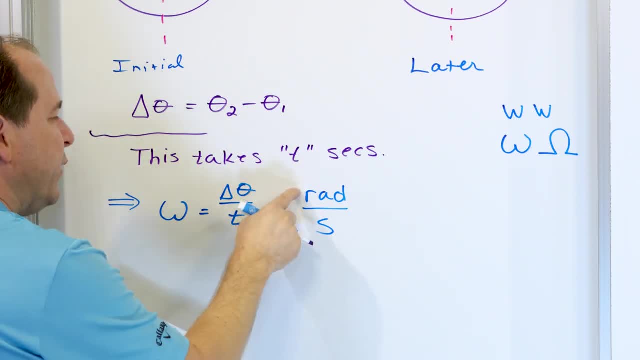 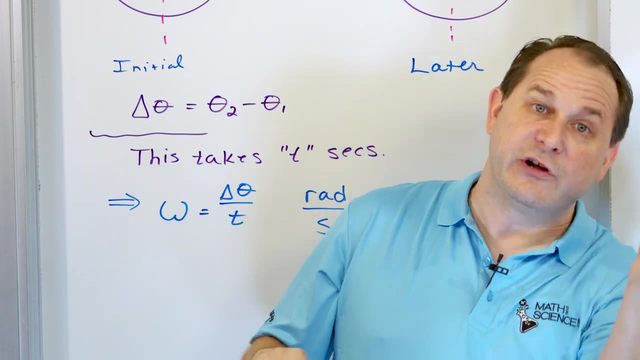 So the unit is radians, And how many seconds did it take? So how many radians per second did you sweep out? If the number that you get is 2 pi radians per second, then that means one revolution of the entire circle, because 2 pi radians is the whole entire circle per second. 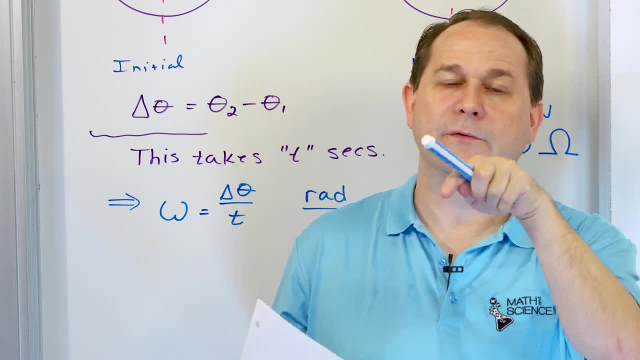 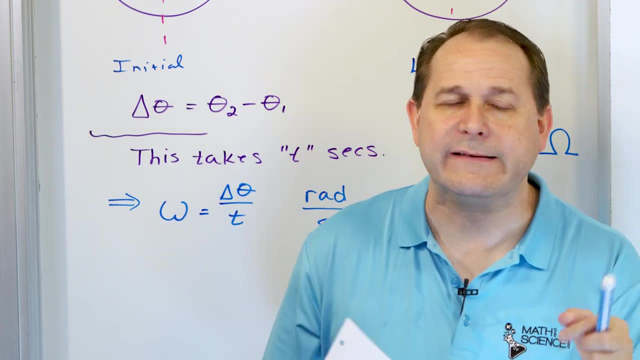 So that's kind of like your baseline: 2 pi radians per second. 2 pi radians per second is all the way around every single second. Any other number of radians per second is going to be slower or faster than that. So it's specifying a rate, but not a rate in terms of distance. 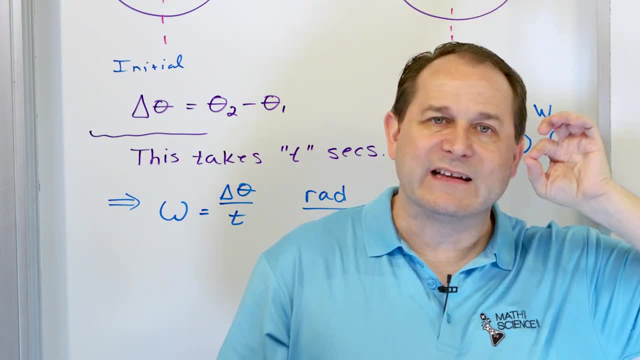 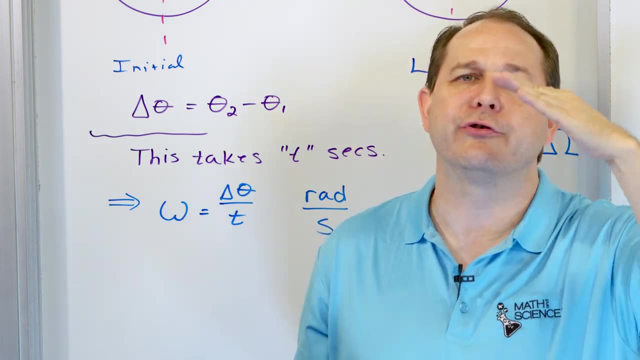 Distance of traveling in a straight line is like meters per second. That's just a linear distance. This is measuring how fast something is rotating by characterizing how much of an angle you're sweeping out every single second, where the angle is represented in radians. 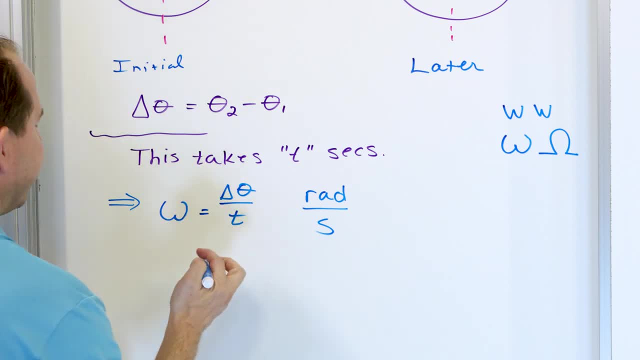 All right. So lowercase omega right here. All right. And we call this angular speed. We don't just call it speed, because when we say speed we always think of meters per second. Angular speed is literally what it says. How fast does the angle change? 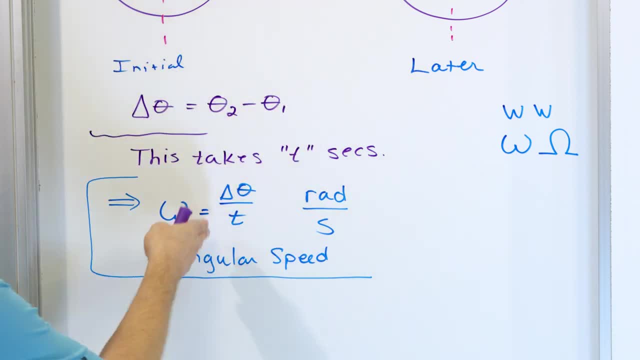 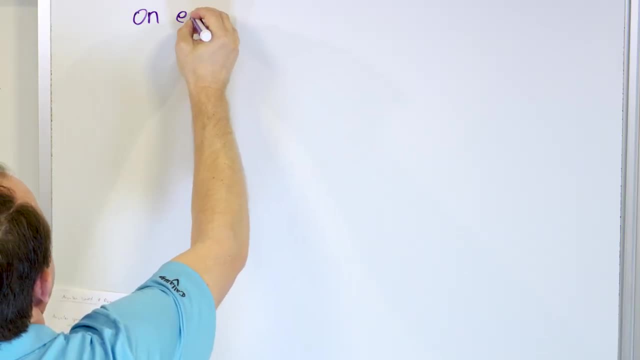 All right, So that's the angular speed, And then what we can do is we can kind of translate this and we can talk about what happens on the edge of the circle. So let's go over here and talk about that On the edge of the circle. 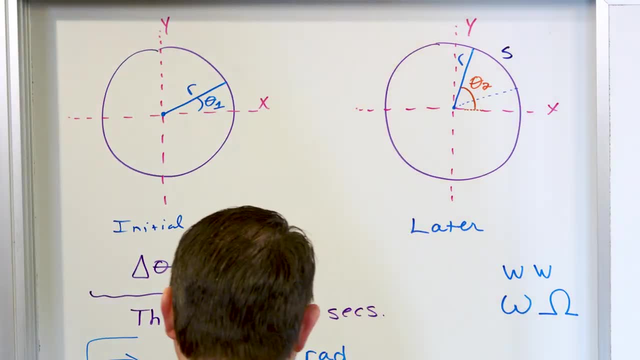 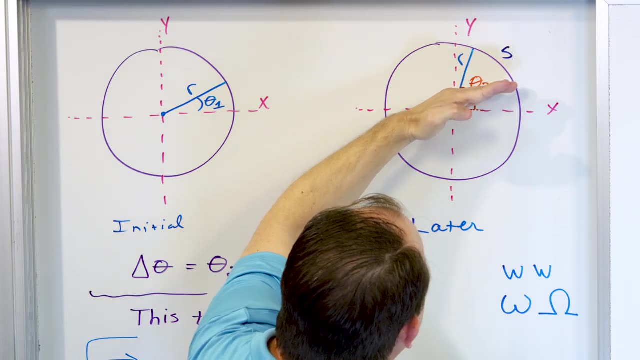 On the edge of the circle. what is happening? So here, what we calculated is how many radians per second we're sweeping out. But notice that as this dotted line travels from initial to final state, the end of it is traveling along the circle. 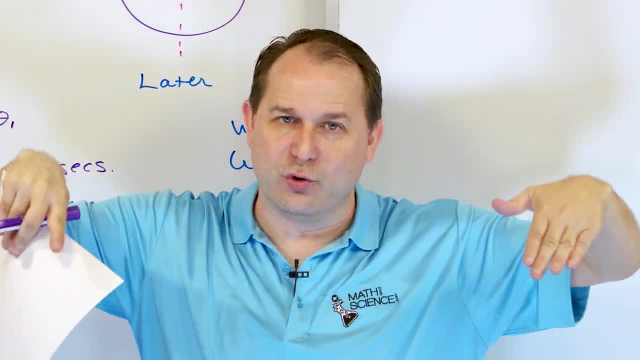 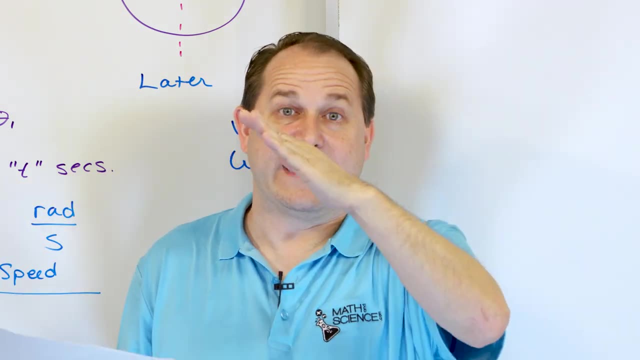 So if you want to think about it, if you think about a old school record player or a photograph player, or if you want to just think of a bicycle wheel spinning, that's fine too, Okay. So if you could visualize the angles, then in radians per second, you can see how fast. 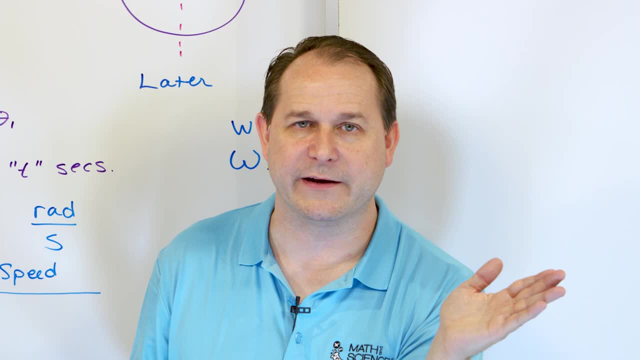 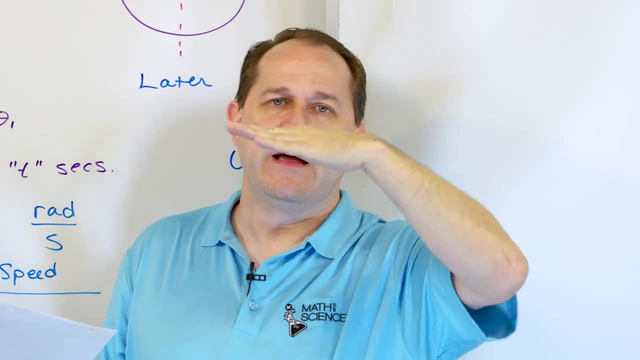 the bicycle wheel is rotating In terms of its angles per second, radians per second. Okay, But if you just fixated your eyes on the edge on the wheel, then you could say that in the same amount of time that we went from state one to state two, the tip of the wheel, the 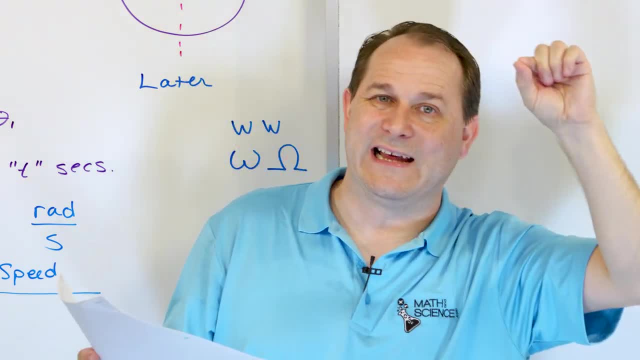 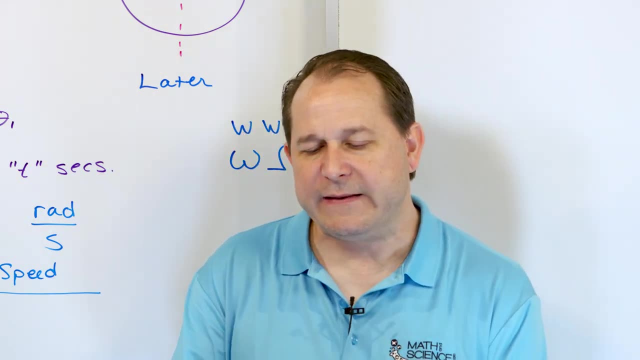 very edge of the wheel along the edge traveled some arc length along its path, the curve path on the edge of the circle per second. That is basically going to be called the rotational speed of a particle on the edge of the circle. So you can think of a record player with a spinning phone. 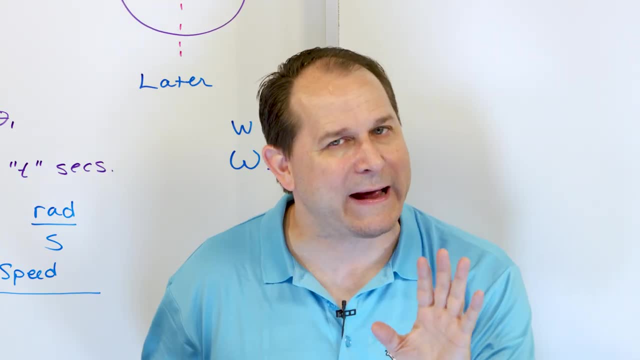 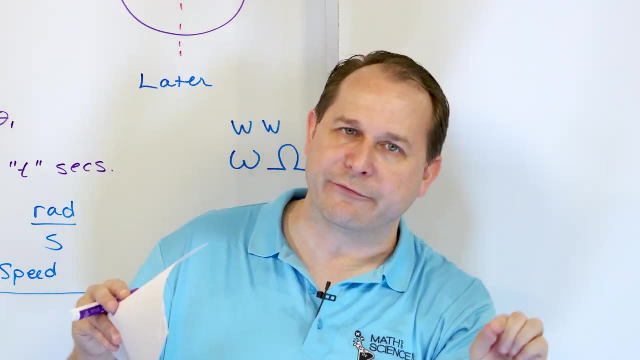 Okay. So if you look at a graph record like this, how many meters per second? and we're not talking about angles anymore. how many meters does a particle on the very edge of the circle travel per second? Or on a bicycle tire, how many meters per second? 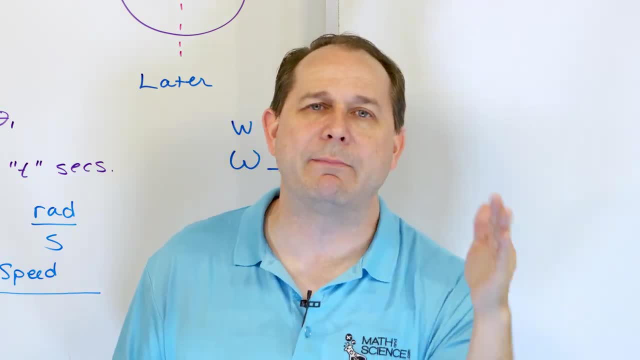 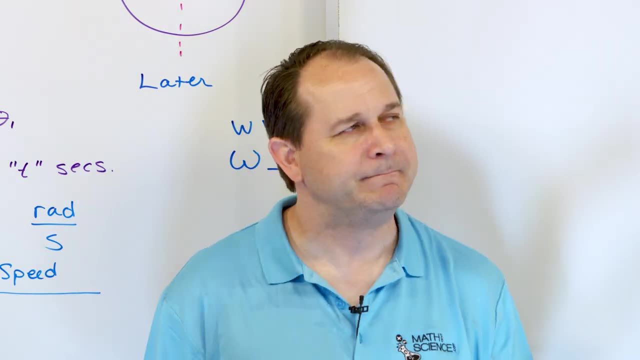 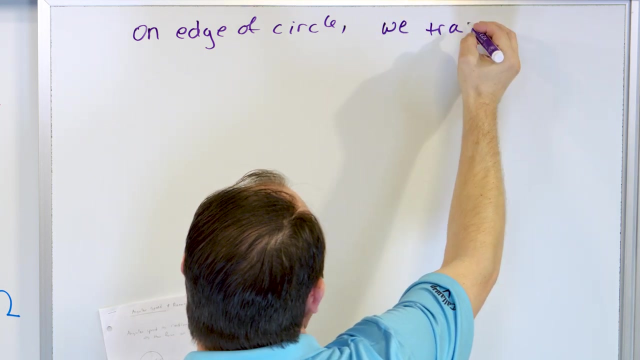 So we're no longer talking about angles, we're talking about linear distance. The problem is because the wheel is curved. it's a meters per second measurement, but it's along the curved edge of the tire, All right. So on the edge of the circle, all right, we travel, and when I say we, I mean a particle. 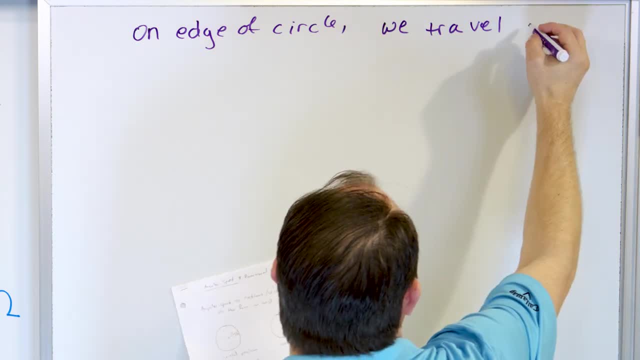 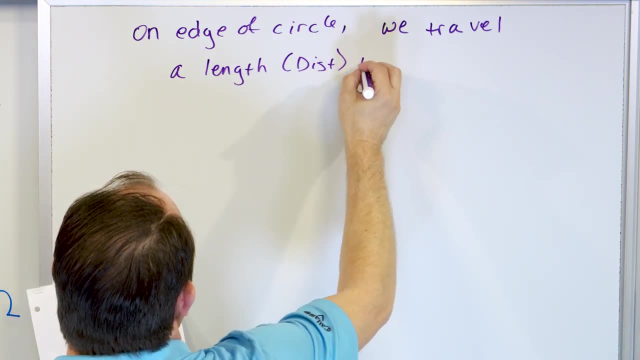 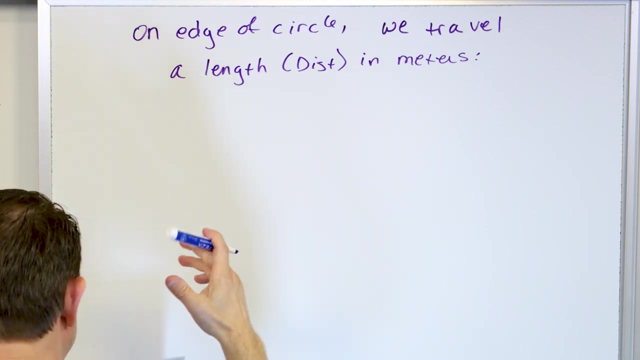 travel. We travel a length which is a distance in meters of the following right. What is the formula for the arc length? We learned that in the last lesson S is equal to r theta. but since we're basically saying it starts from here to here, we're. 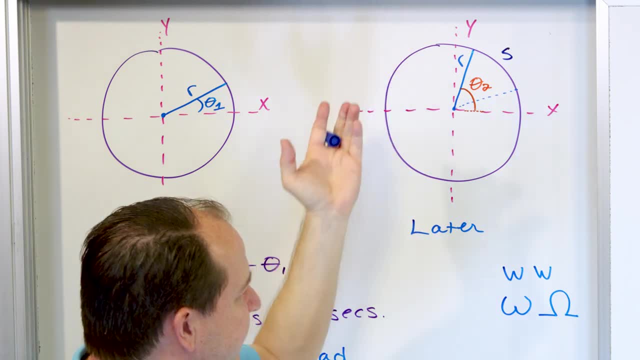 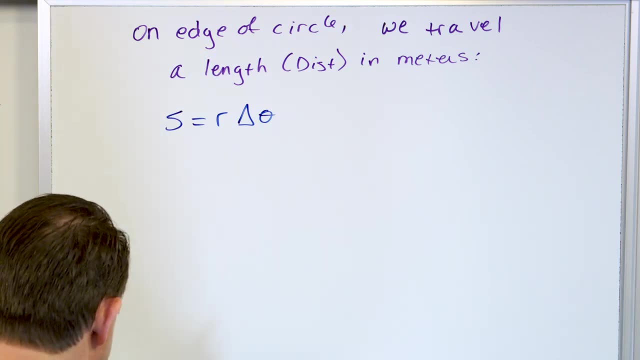 really calling this angle here delta theta. That's what we're really calling it. We'll just call it delta theta, which is just r Times the angle in radians that it sweeps out. All right, So the speed on the edge is the following: 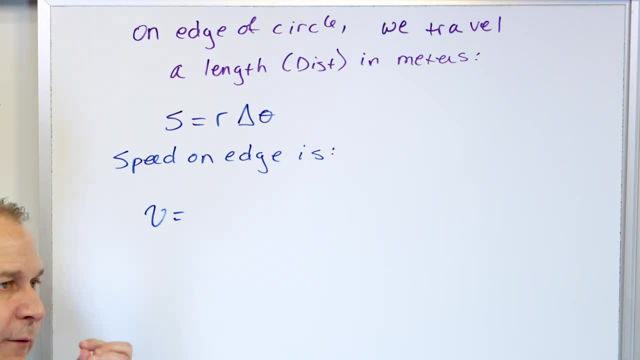 What is any velocity Distance divided by time? right, If I travel five meters straight line distance, five meters in 10 seconds, it's distance divided by time. Any velocity in meters per second is just distance divided by time. We're just saying that the particle is sweeping out along the edge of a circle, a curve distance. 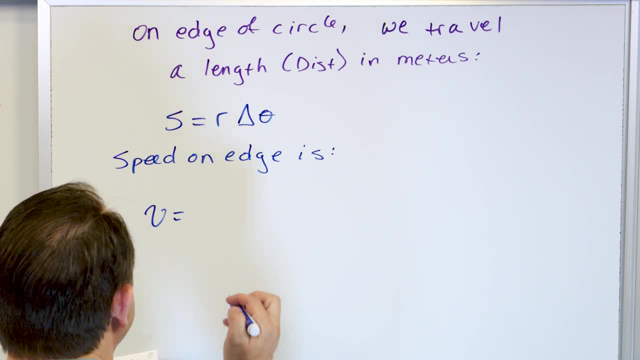 that we call the arc length, But still it's distance divided by time, But the distance along the edge is just the arc length divided by however many seconds it took to actually sweep that out, But we already know what the arc length is. 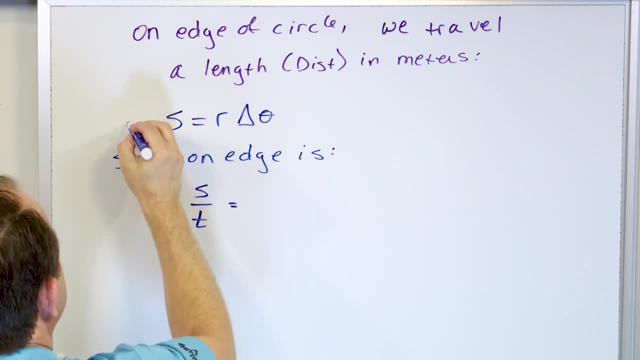 It's r times delta t, So we'll just replace this, We'll go and we'll put this in here, right here, We'll say: r delta theta divided by t, All right, And then what we can do is say: well, wait a minute. 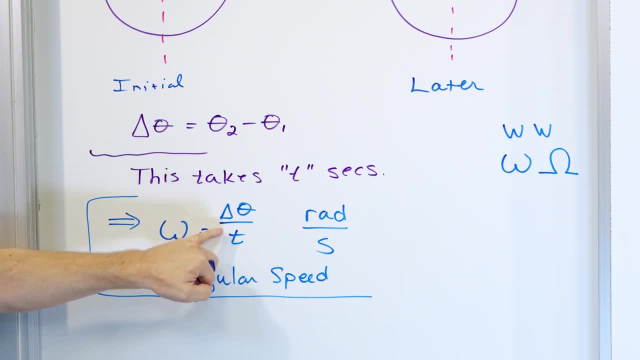 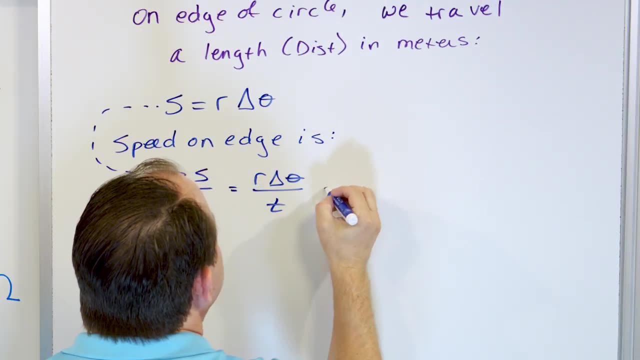 We already know that omega, the angular speed, is equal to delta, theta over t, which is the angular A rotational speed angle divided by time. But we have that right here, So we could say it's r times omega. So what I'm going to do is I'm going to circle this. 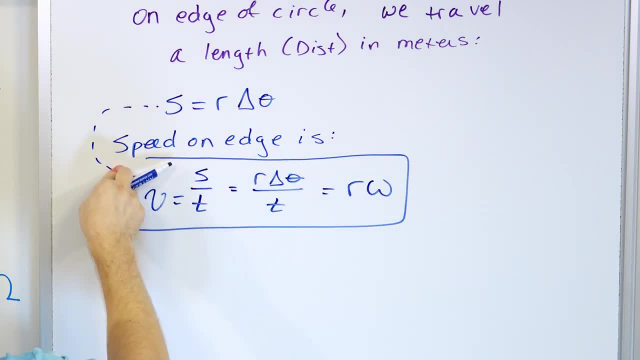 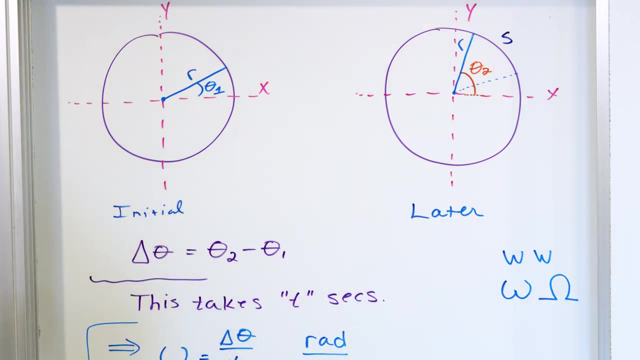 I really wish I'd use a different color. Sorry about that. I guess what I'll do is take this away and put a little arrow right here and just make it a little bit cleaner. So we have transitioned from learning what an angular speed is how many radians per second. 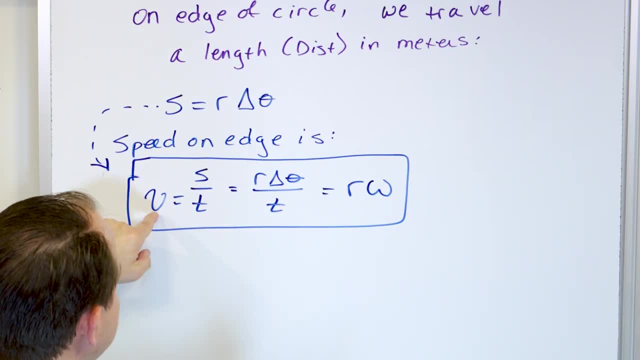 something is rotating, to trying to calculate the velocity of a particle on the edge of a circle. So all you do is you say how far does the particle on the edge of the circle travel? That's the arc length traveled divided by the time in seconds. This is meters per second. That's the. 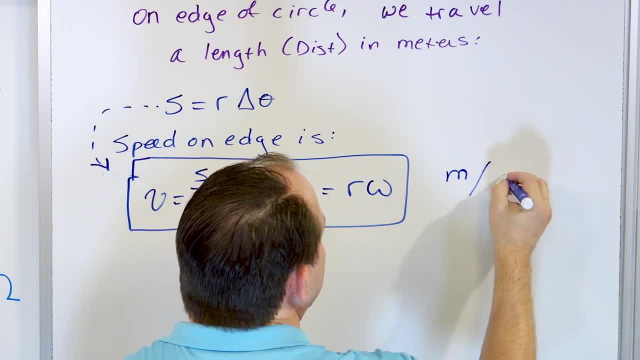 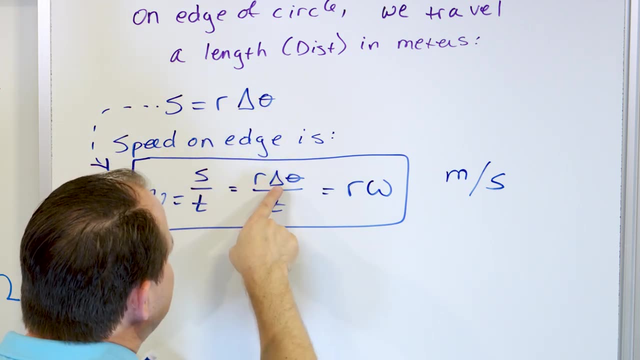 unit that you would get here. So this is meters per second is the answer you would get here, But we already know how to calculate the arc length. It's the radius of the circle times, however many degrees you rotate through. So we just substitute that in So you can use this. 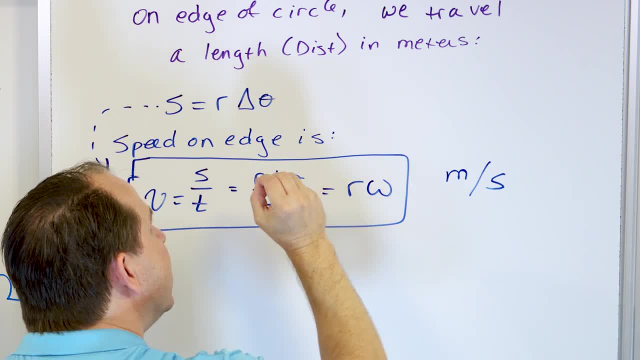 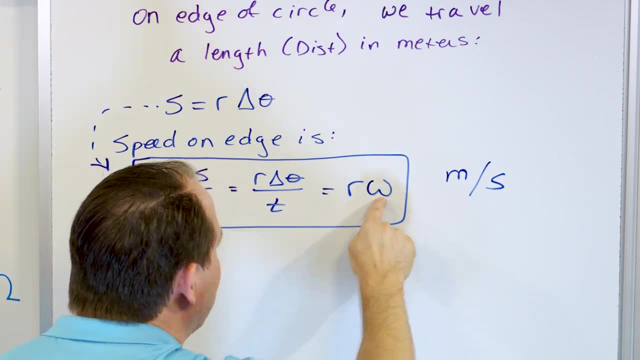 equation if you want. But then we realize that this quantity, theta divided by t or delta theta divided by t, is radians per second, which we called omega before. So you could say that the speed of the particle on the edge is the arc length divided by the time. That's fine, Or you? 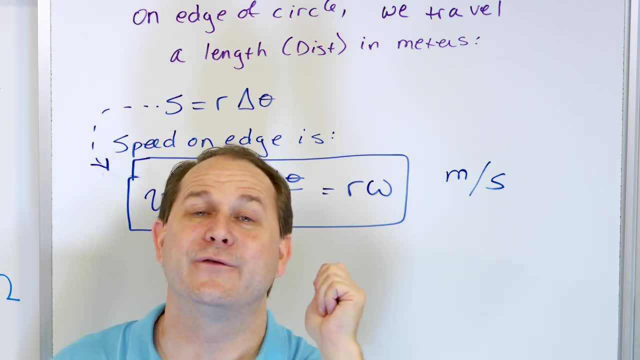 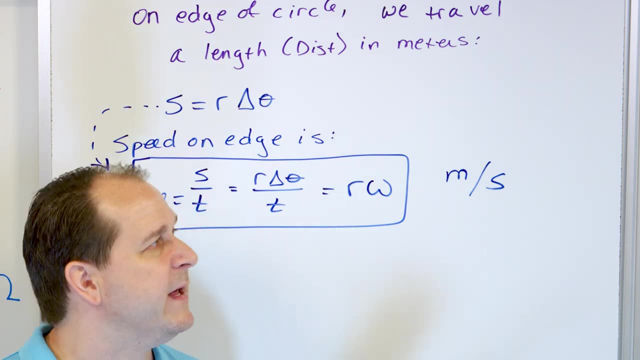 could say it's the radius of the circle multiplied by the angular frequency. So many times in math and science and physics there's different ways of solving a problem. If you're given the arc length, then you can easily calculate it And you know how long it has to be. 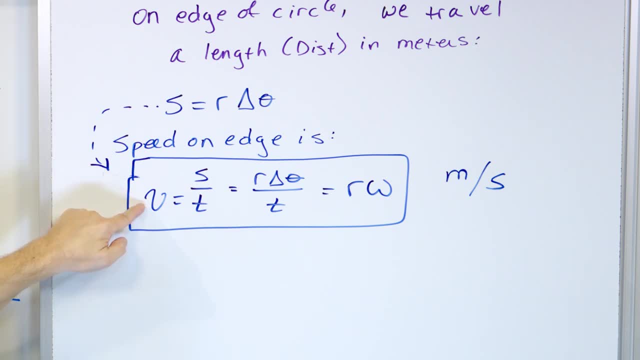 But if it happens in seconds, then just use this equation to tell you how fast a particle on the edge of the circle is traveling. But if, instead, you're given the angular frequency in radians per second and you're given the radius of the circle, this would make a lot more sense to use. 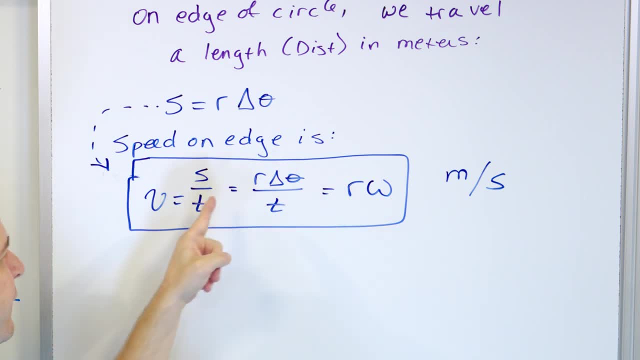 because you're already given that information. So it's not so much that this is better than this or this is better than this or this is better than this. They're all equivalent. That's why there's equal signs in there, And it's just going to depend on what problem that you have here. 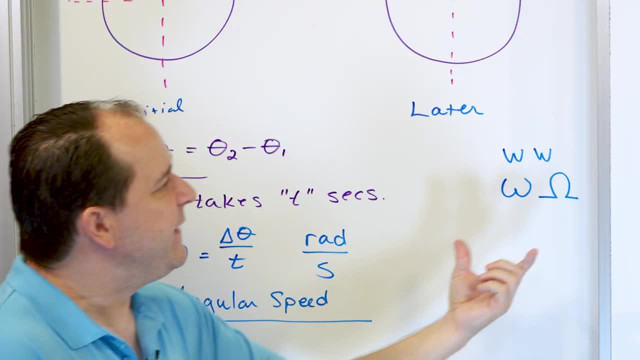 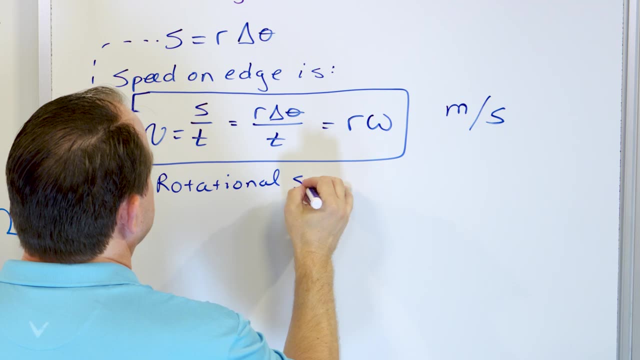 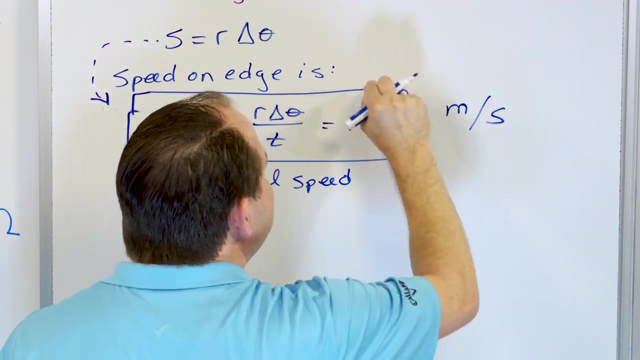 So this thing over here was called angular speed. This thing is called rotational speed. Basically it's the speed that a particle is traveling along the edge of a rotating circle in meters per second traveled around the rim of that circle, This is more of an. 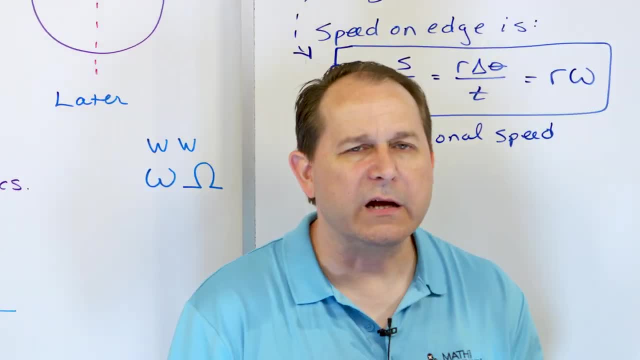 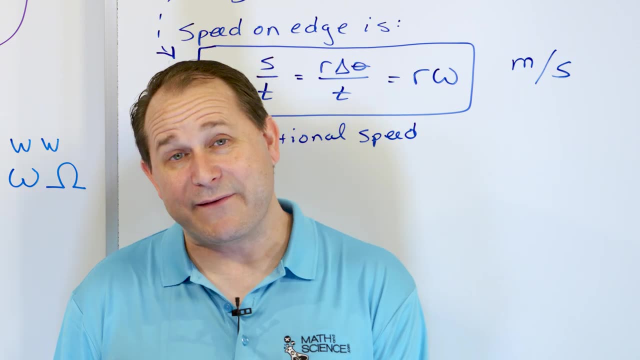 angular measure. Now here's a dirty little secret: In some problems, when you're given exactly what you need, you'll just use these equations. That's why I'm deriving them for you and trying to tell you what they are. However, a lot of times, when you're actually solving problems, you don't really 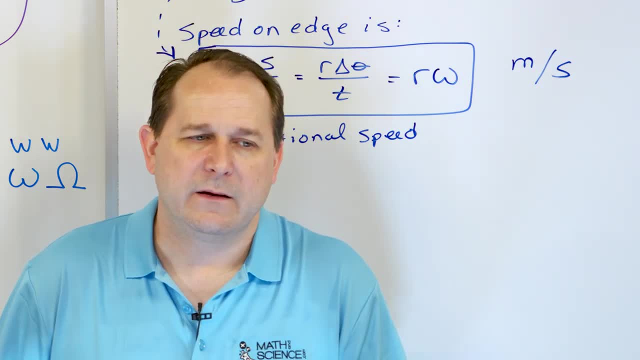 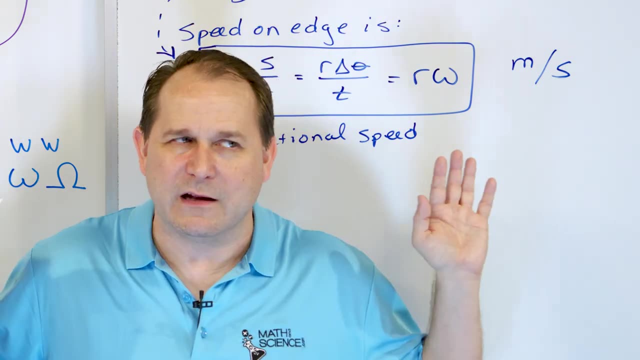 need to use these equations too much. I went through the exercise of deriving it for you so that we could kind of get comfortable with it. But really when we solve a lot of problems you can a lot of times forego using these equations, as long as you know what you're. 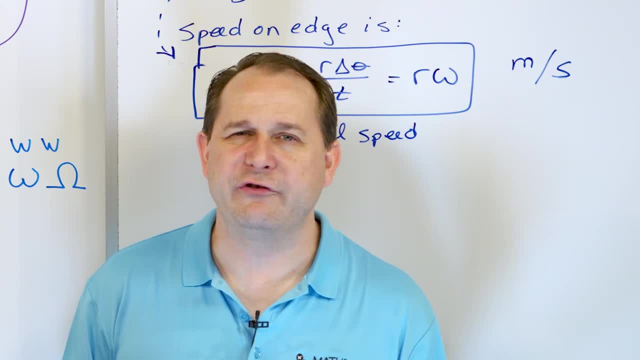 doing. So what I'm going to do when we solve the problem- at least the first one- is I'll solve it two ways and show you kind of what's going on. So let's take a look at problem number one. It says: 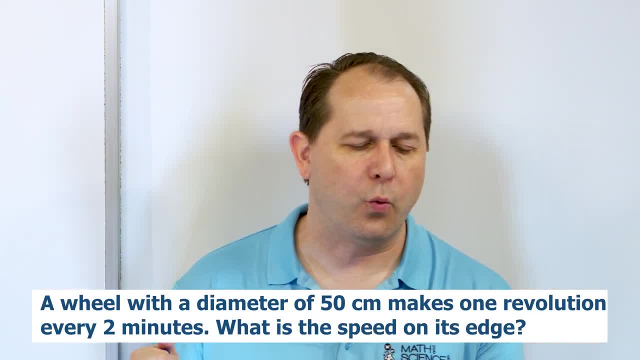 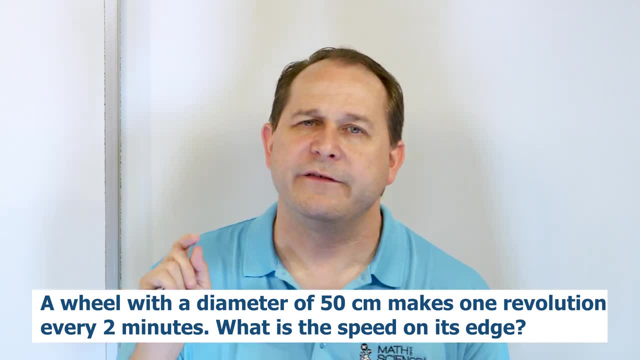 a wheel with a diameter of 50 centimeters makes one revolution every two minutes. What is the edge of the wheel in centimeters per minute? So that's the crux of the question. They even give us the units here. What is the speed on the edge of the wheel? So that's not an angular speed. They 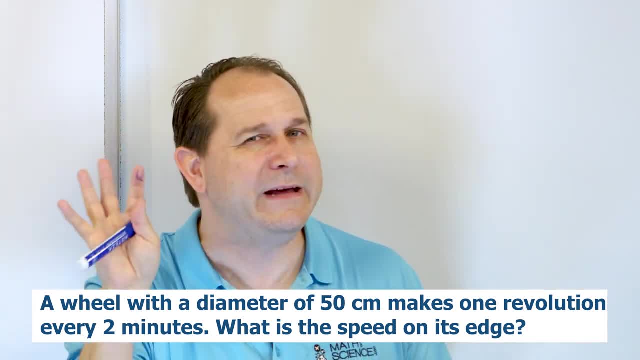 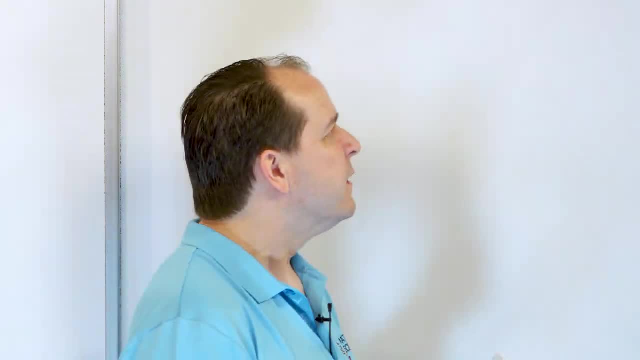 want to know how many meters per second the edge of this wheel is traveling, but it's not meters per second. They actually tell us they want it in centimeters per minute, but still it's a distance per unit time on the edge of the wheel. So to start out it's going to be much easier, as always, to 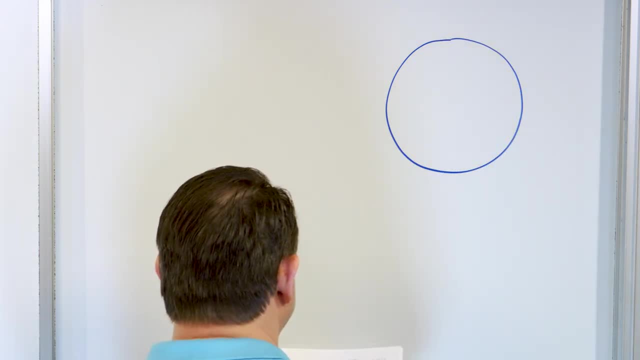 just draw a picture, And we always need a circle for motion involving a circle, So we'll just draw it there Now. it says a wheel with a diameter of 50 centimeters makes one revolution every two minutes. What does that mean? It's a circle with a diameter of 50 centimeters, So that means that. 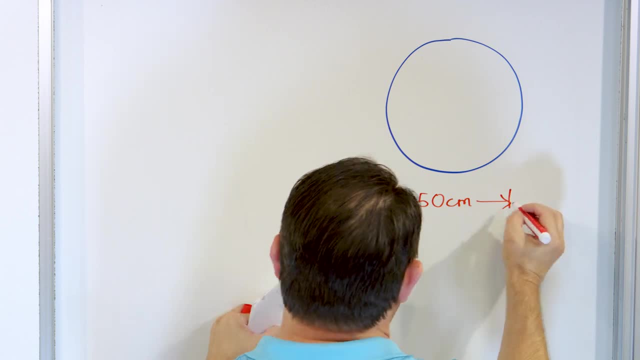 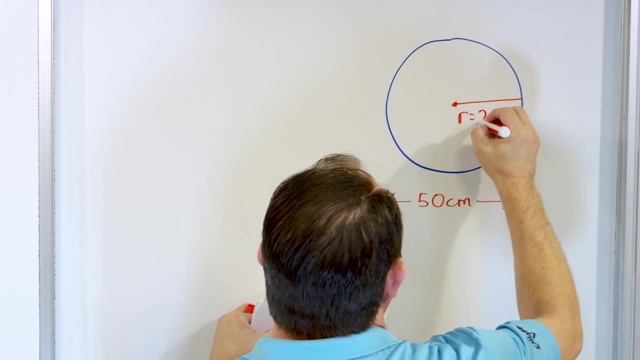 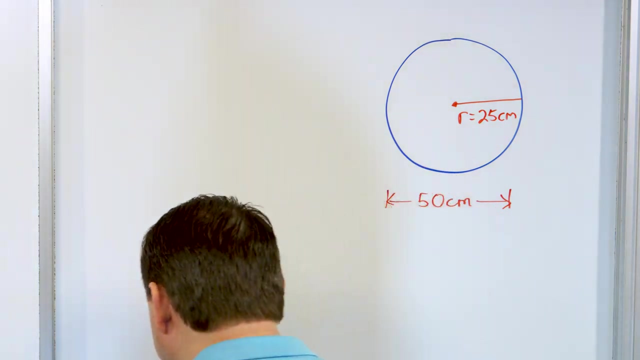 this is 50 centimeters, Like this, And that means that the radius which we know we're going to need is going to go to here, and that radius is 25 centimeters, and that's just the diameter divided by two. Now, what we're asking in this problem is if you had a particle here and this thing is. 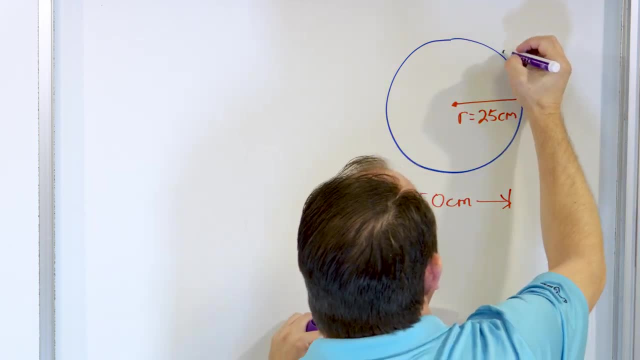 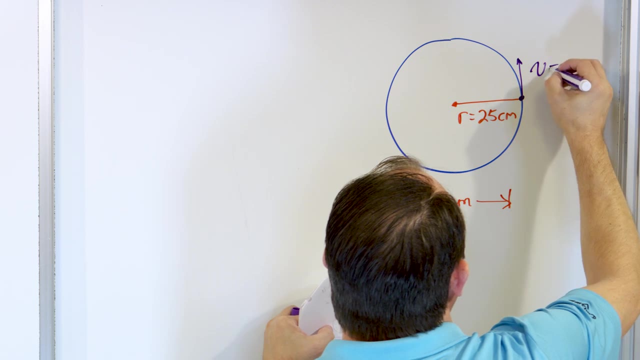 rotating, which it is rotating. it's going around and around and around. this thing is traveling a a curved path, So at any instant of time its velocity is kind of tangent to the circle. We want to know what is this velocity in centimeters per second of a particle traveling? 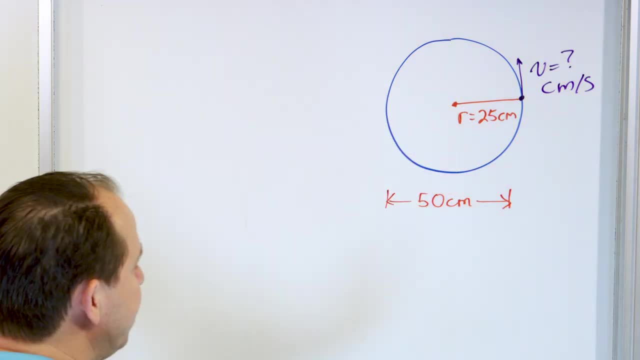 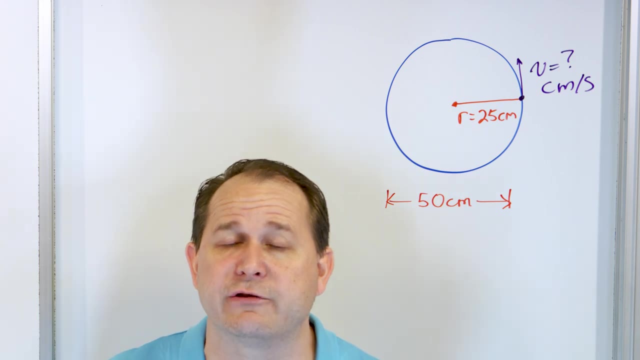 along the edge of a circle. All right, so there's a couple of different ways you can proceed. What I want to show you is the power of unit conversions. A lot of times you can solve a lot of unit conversions without even knowing any equations at all. Let's read the problem one. 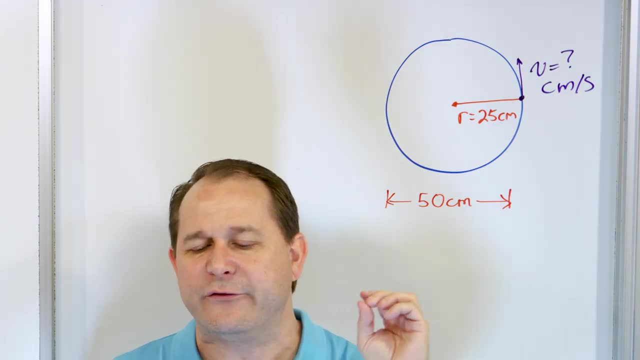 last time A wheel with a diameter of 50 centimeters we got that makes one revolution every two minutes. What is the speed on the edge of the wheel in centimeters per minute? So let's pretend we don't know any of these equations that I've already derived in the previous boards, And let's 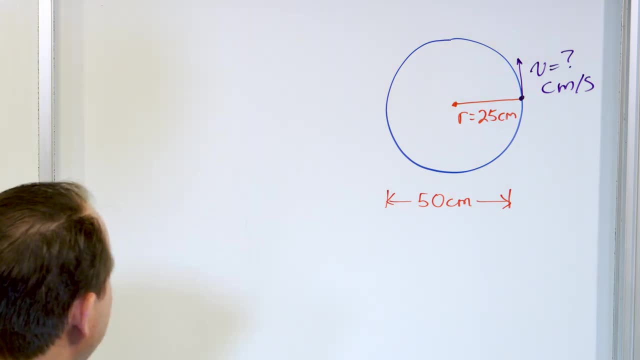 just say: we don't even know them, Let's just proceed. This wheel is rotating one revolution every two minutes. So what we do is we set this up as a conversion factor, one revolution per two minutes, And we draw our conversion factor. 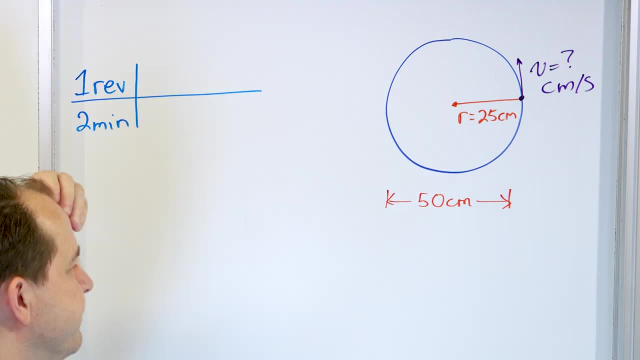 Like this. This is perfectly fine to do. You can set up any equivalence in a conversion factor like this: You know that there are one dozen is equal to 12 of something. That's a conversion factor. You know that there are 1,000 meters in a kilometer. That's a conversion factor, You know. 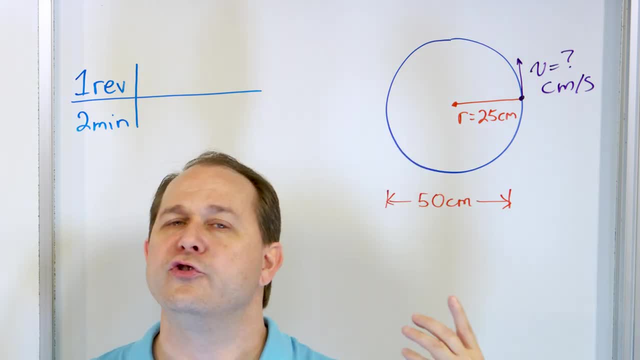 that there are two pi radians in one revolution of a circle. You could write that as a conversion factor: Any two things that are equivalent, even if they're not like standard units that you are thinking about like liters and things, if they're. 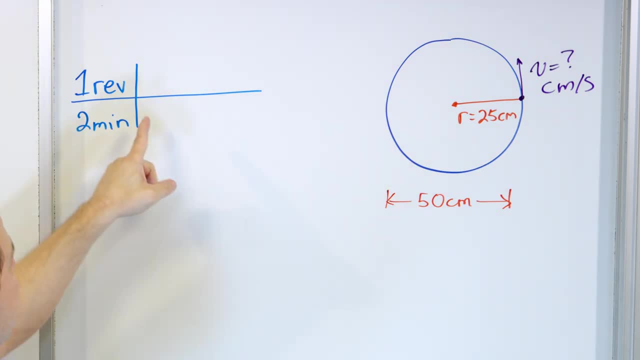 equivalent. you can write that as a conversion factor. So we don't typically think of the word rev to be a unit, but it is a unit. A revolution is just the idea of going all the way around one time. So even though it's not a typical unit that you think of with unit conversions, it is perfectly legal to put in here, because we know that the quantity one revolution is equal to the time of two minutes. One revolution per minute, just like you could put meters per second here. All right, Now we have an important part of the problem. 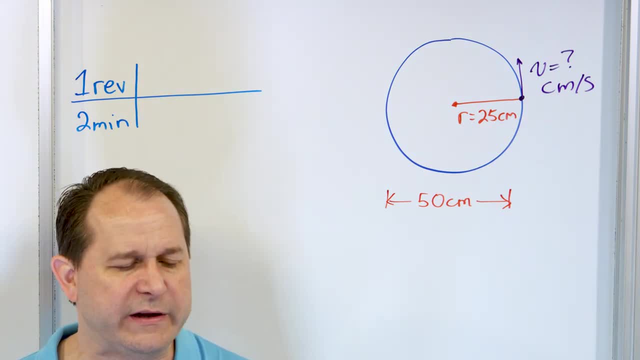 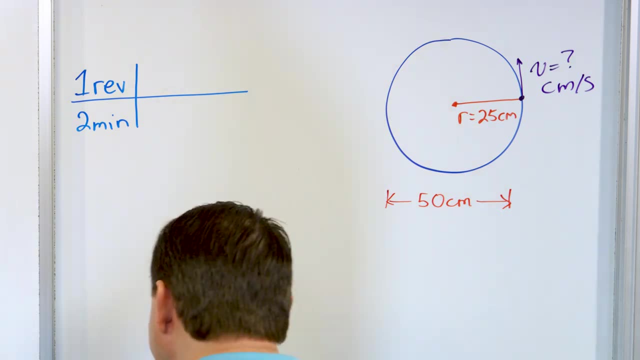 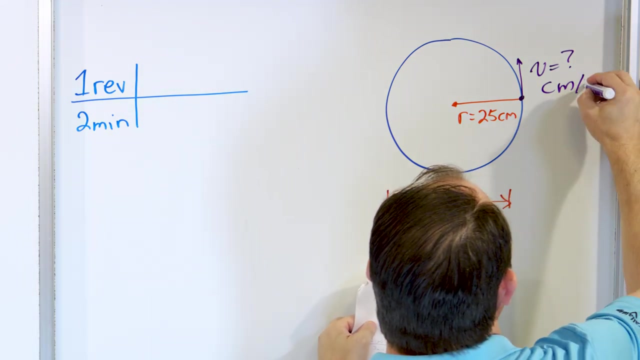 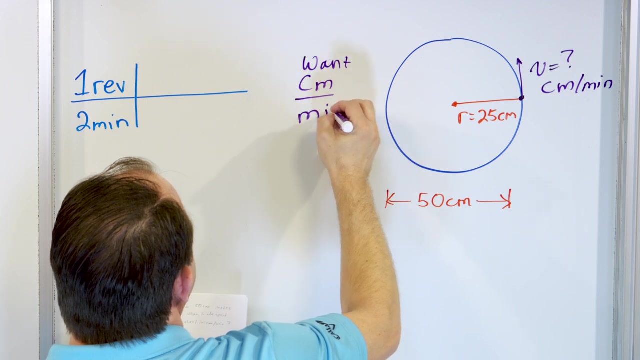 All right. Then it says: what is the speed on the edge of the wheel in centimeters per minute? So all you want to do is you want to figure out how to get from this unit right here into- and I already made a mistake- centimeters per second. We don't want centimeters per second, We want centimeters per minute. Sorry about that. So we want centimeters per minute, And all we have to do is multiply or divide to get to centimeters per minute. Now look at this. We already have minutes on the bottom. 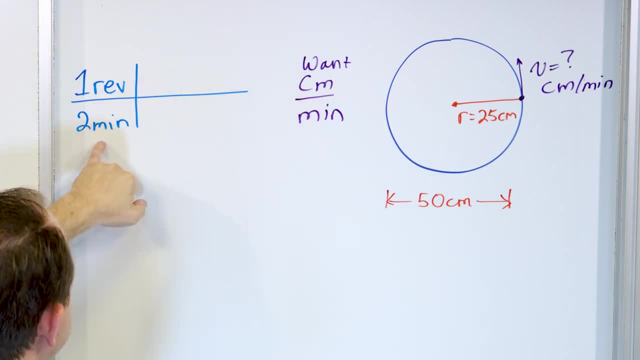 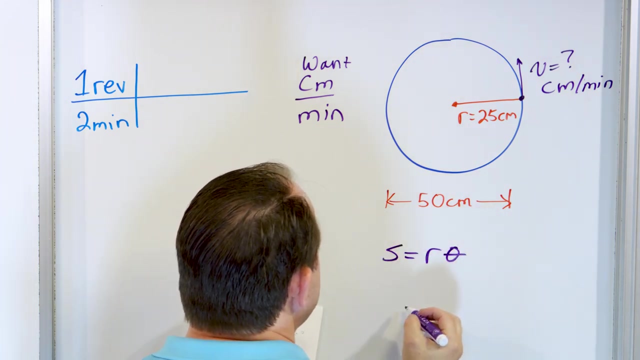 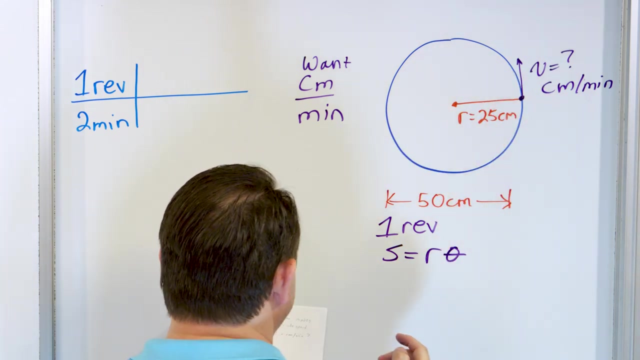 So actually half of the unit is already done. We already have minutes on the bottom. The problem is the revolutions. We want to figure out a way to change revolutions into centimeters, Revolutions into centimeters. How do we do revolutions into centimeters? Well, we already have an arc length. formula S is equal to R times theta. And we can say: well, let's take a look at one revolution around this circle. Right, How far would it be for one revolution to go around the circle? What would the arc length be? The arc length would be the radius, which is 25, which is in center. 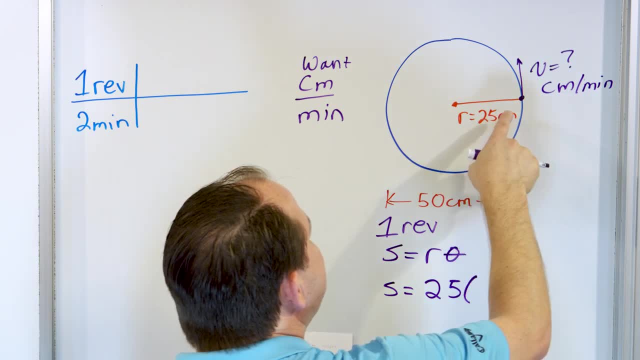 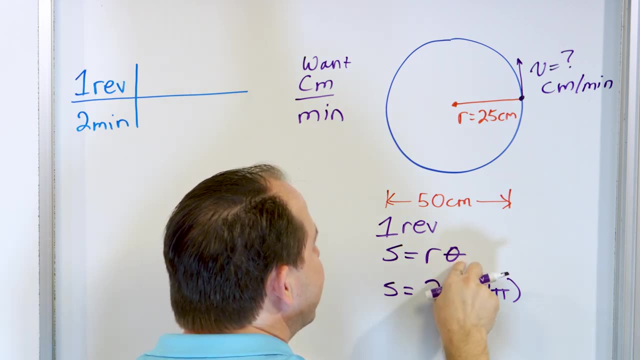 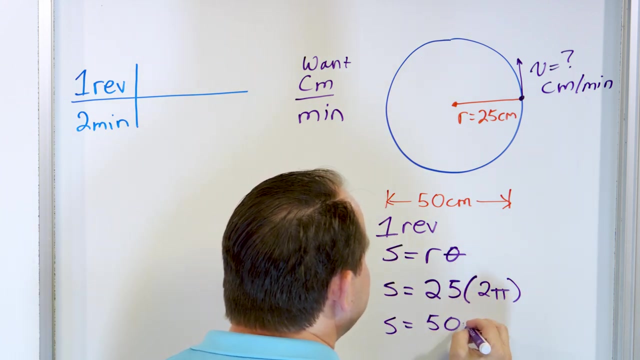 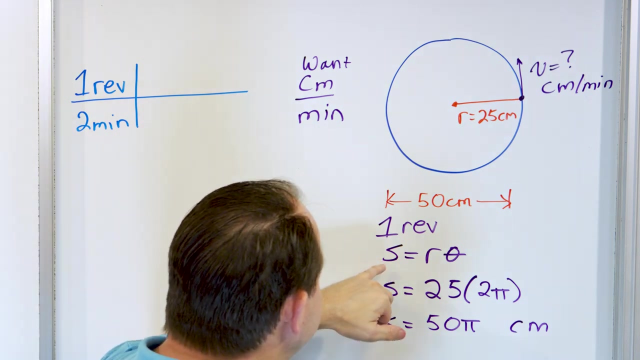 And for one entire revolution it would be going all the way around, which would be 2 pi radians. So we put a distance unit in here for radius and we put an angle in here for radians. So this is centimeters right here and this is radians right here. So 25 times 2 is 50. But then we still have to multiply by pi. What unit are we going to have here? This is centimeters Right, Because this is essentially the arc length going all the way around. Now what's another way to figure out the circumference of a circle? That's what you're going to have to do. 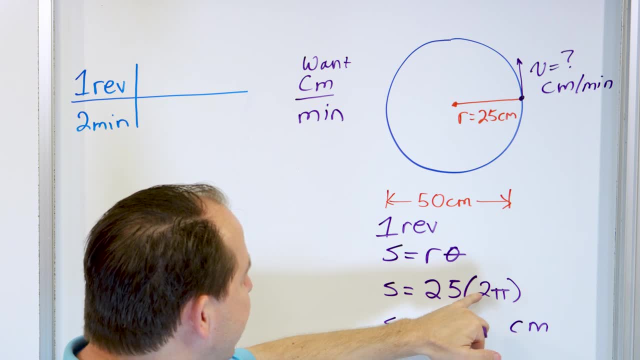 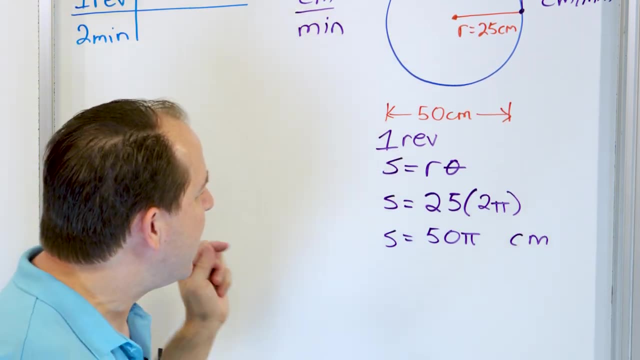 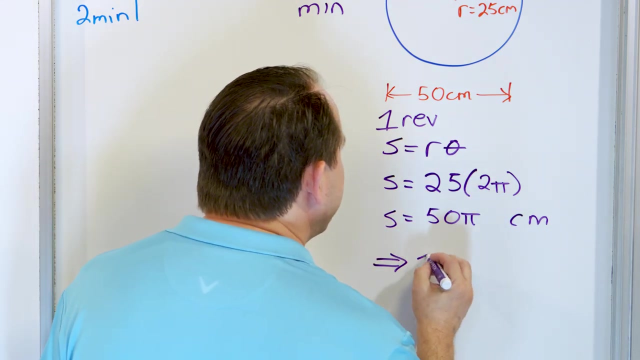 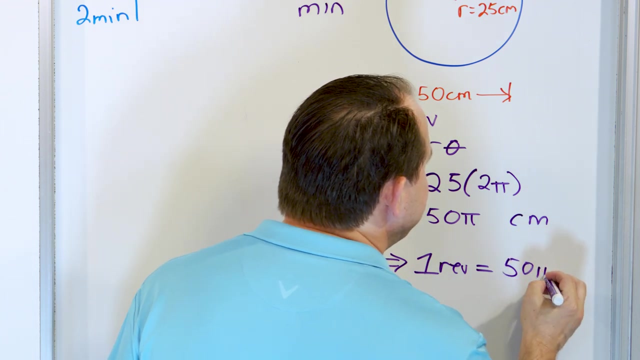 You're calculating 2 pi R. All we've done is multiply 2 times pi times R, So I called it arc length, all the way around. but it's exactly the same thing as finding the circumference of that circle, And what we have figured out is that the circumference of the circle is 50 pi centimeters. Another way of saying that is we've made the equivalence that one revolution of the circle is equal in distance to 50 pi centimeters. This is another conversion factor. 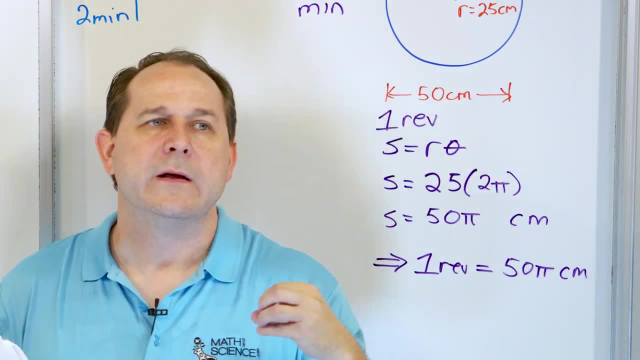 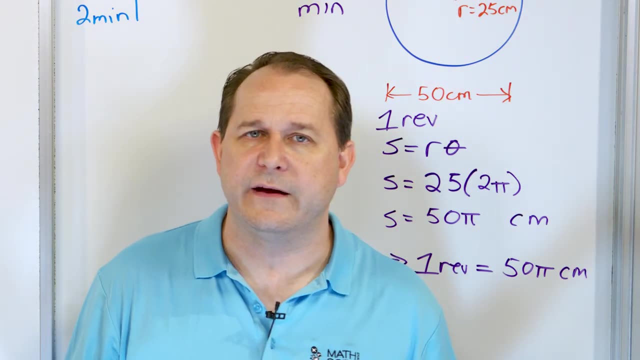 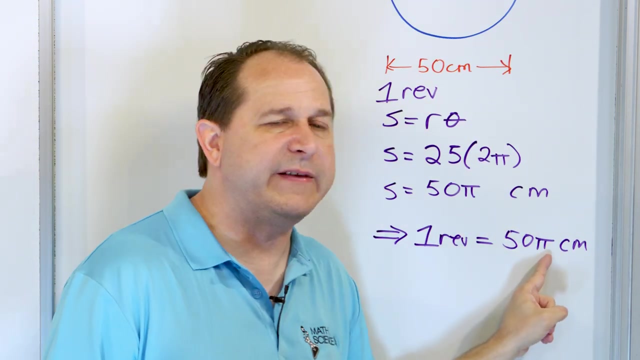 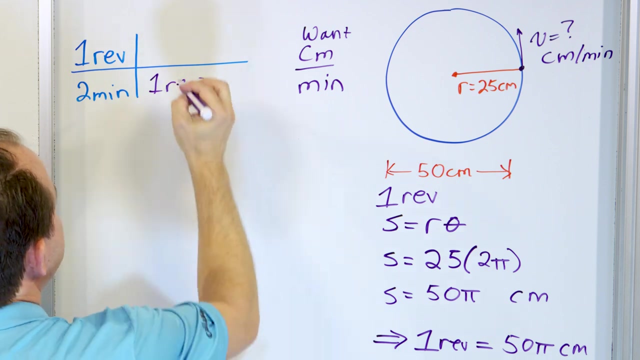 When we calculate the circumference around the circle without saying it. what we're implying is that what we're saying is one revolution around the circle is equal to whatever the distance is, And it's an equivalence, It's a conversion factor. Just like one revolution takes two minutes, we're saying now, one revolution is also this unit of distance. So what we can do is we can write it like that: We can put one rev on the bottom and we can put the 50 pi centimeters on the top. Why did we write it like this? 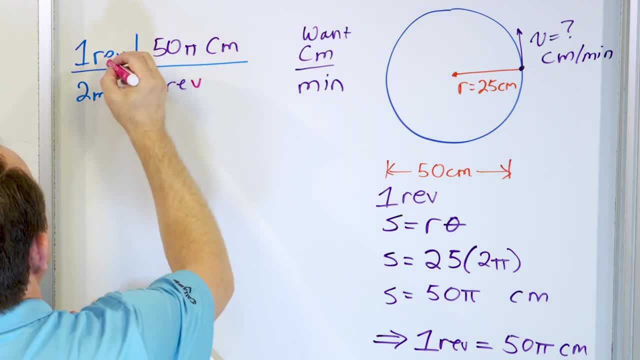 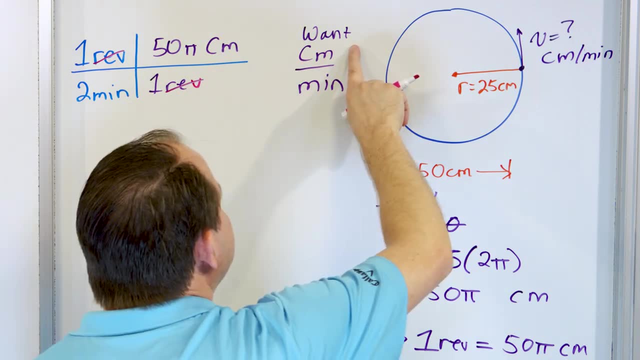 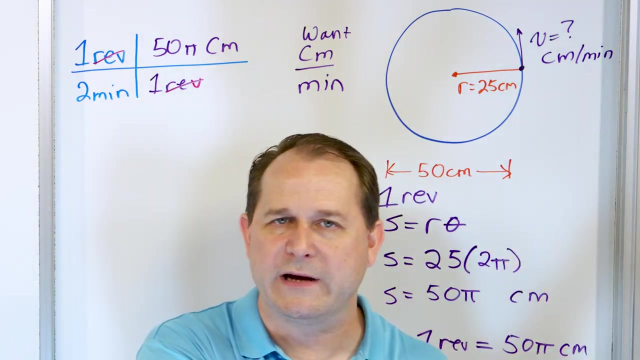 Because this should be say rev. Sorry, Rev will cancel with rev, which is what we always do when we set up unit conversions And we have a centimeter on top and a minute on the bottom, This is the unit we want. So you see, we didn't actually use any of the equations. All we did was start what we know and say: what unit do we want to get? How do we get there? logically, using valid conversion factors. 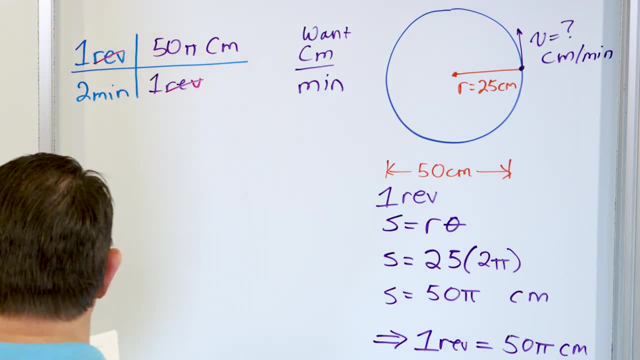 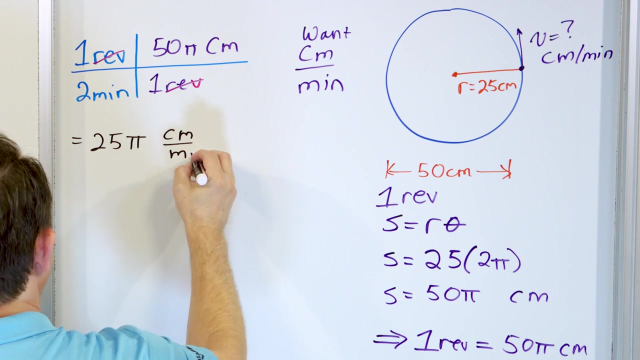 So what we do is then we say: 1 times 50 pi is 50 pi, So what you're going to get is 50 pi. So what you're going to get is 50 pi divided by 2, which is 25.. So you have 25 pi and the unit is centimeter per minute, And you can approximate this. or when you take 25 multiplied by 3.14,, 78.5 centimeter per minute. 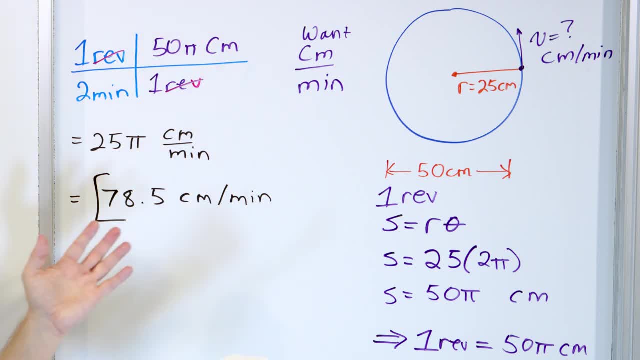 Now this is the answer to the problem. Now, this is not probably the way most people would think to solve this problem, to be honest with you, because I just gave you all these equations. We didn't really use them right, But you actually did use them, It's just that we did it in a totally different way. This is extremely powerful. You didn't even know what the equations were, You just knew what unit you were trying to get to. 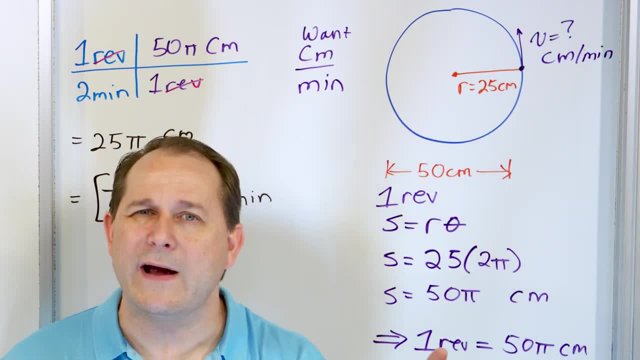 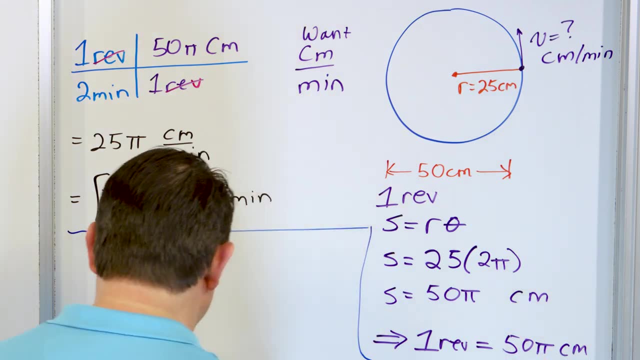 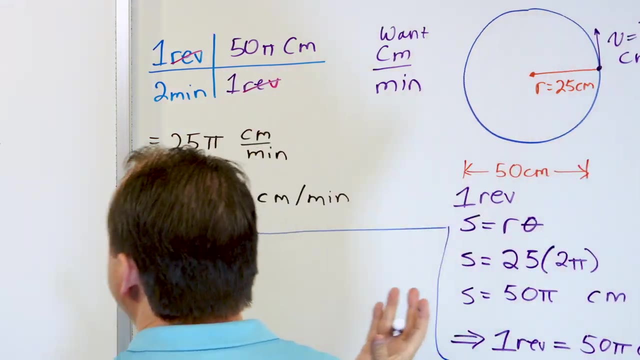 And, of course, you knew the arc length to tell you the circumference all the way around. And that's how we did it. Now let's go back and try to solve it a second way, using the equations that we actually have. All right, so what this problem asks for is what is the velocity of a particle on the edge of the circle in centimeters per minute, And we actually have an equation for that. 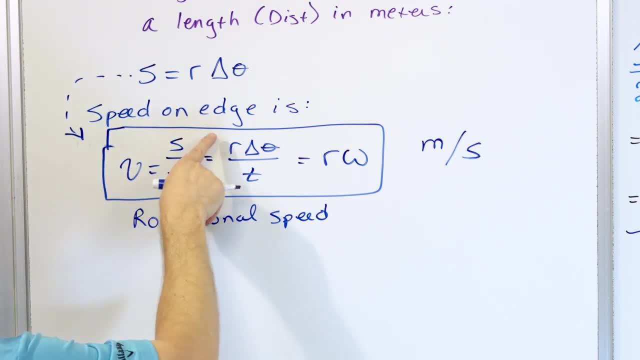 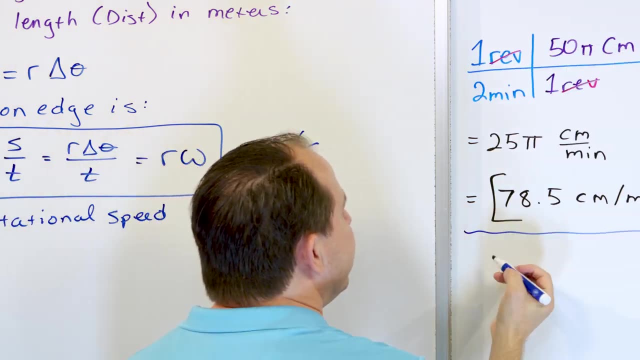 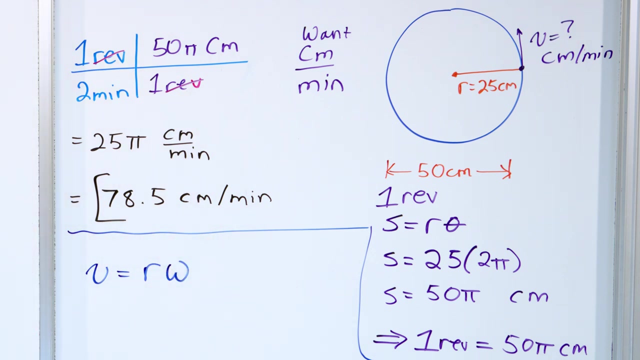 It's some arc length multiplied by time or divided by time. which is this over this, which is also the radius of the circle, times omega. So let's just use that V is equal to r omega. So we could blindly say the velocity on the edge of the circle is equal to the radius of the circle times the angular speed that the circle is rotating at. This is going to convert it into meters per second. 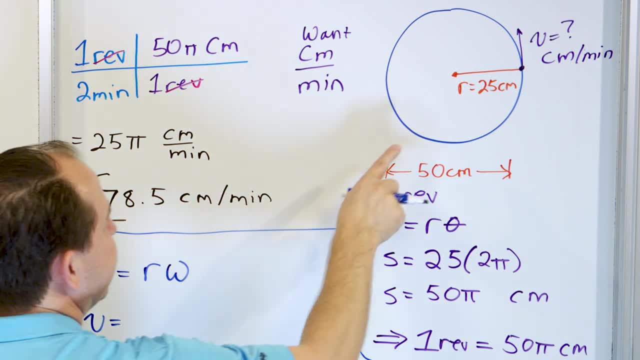 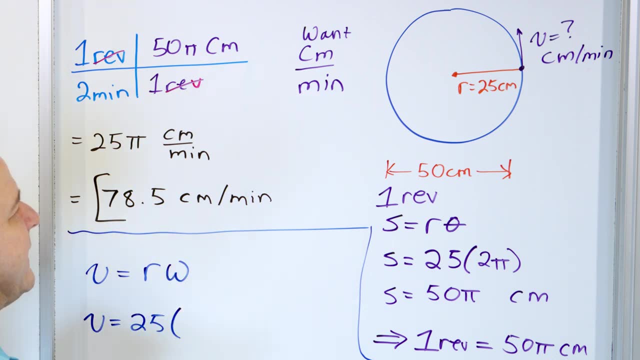 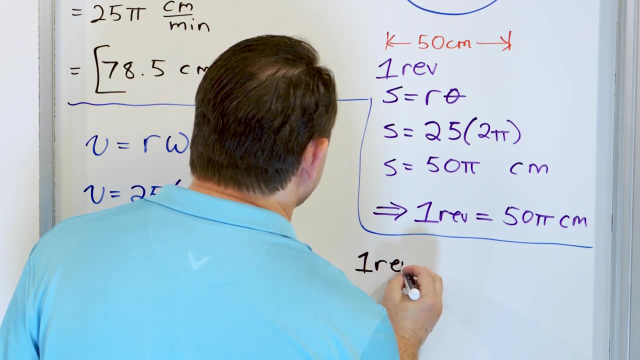 So what's the radius of the circle? Well, the radius is given to us as 25 centimeters, So I'll put 25 right here, right? And what is omega Radians per second? Now, that's the trick. I don't actually have that for this problem, But I do know that I can go down here and say that I'm traveling one rev every two minutes. 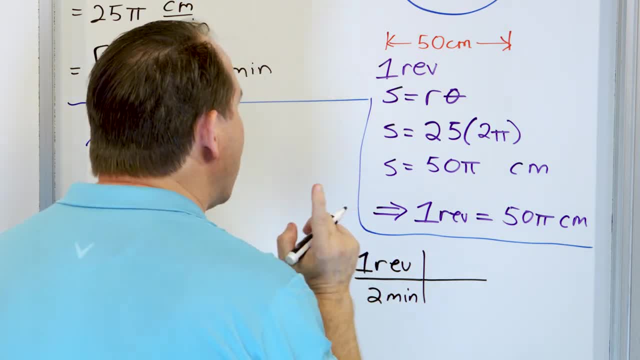 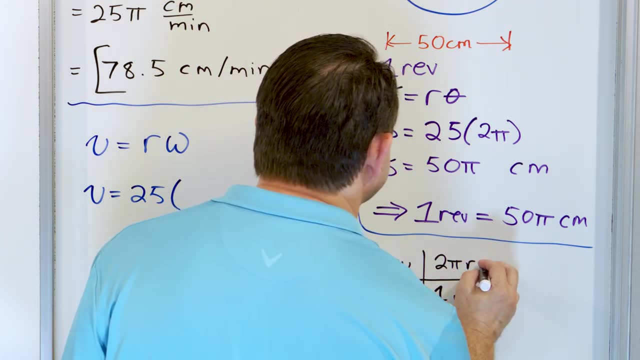 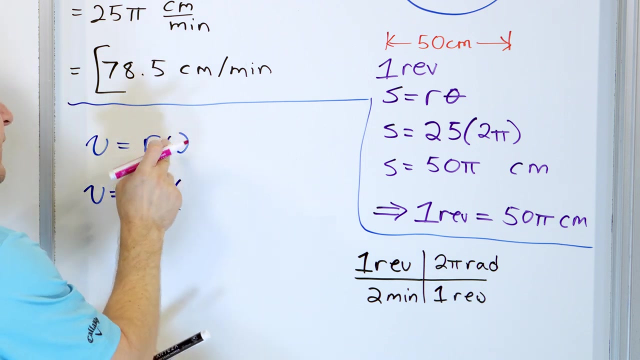 One rev or one revolution every two minutes. But I also know that. I know that one revolution is exactly the same as two pi radians. Why am I equivalent? why am I bringing radians into it? Because, in order to use this equation, I need radians per second. 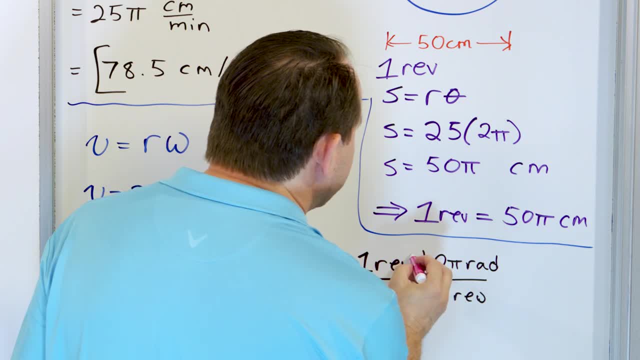 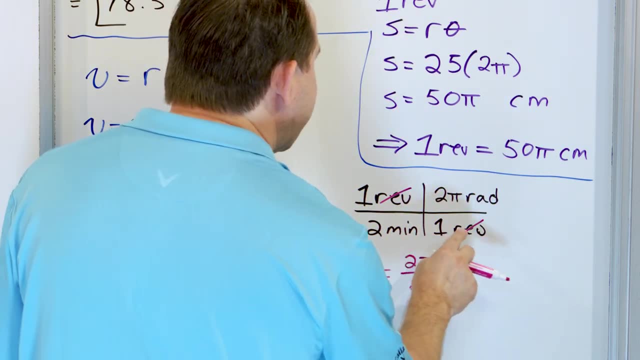 I need some radians per unit time, In this case radians per minute. So what I'll do is I'll cancel the revs And what I'm going to get here is two pi on the top, But I'm going to be dividing by two on the bottom And the unit is going to be radians per minute. 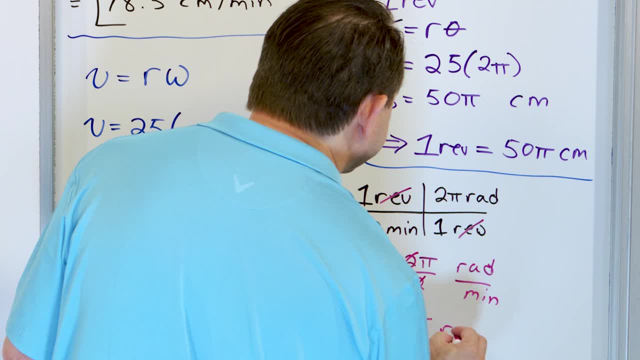 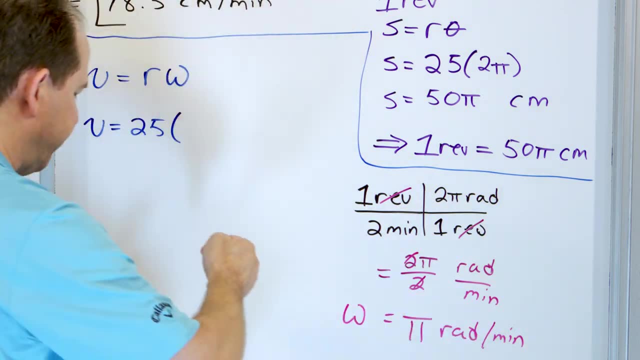 And when you cancel the twos it's just going to be pi radians per minute. So what we have figured out- because this is a unit of angular speed, angular speed is pi radians per minute. So every single minute that goes by it's going to be pi radians per minute. 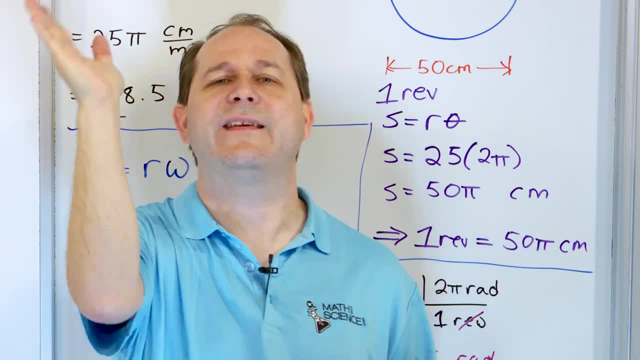 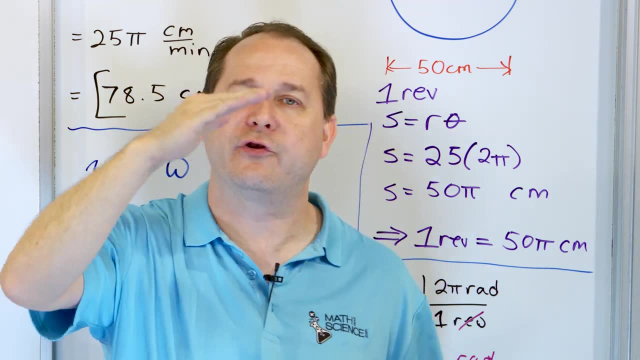 So every single minute that goes by we travel a half circle, because pi radians is halfway around the circle. Two pi radians is around the whole circle. So every half minute it goes another half of a circle. That's telling you how fast, in terms of angle, the thing is rotating. 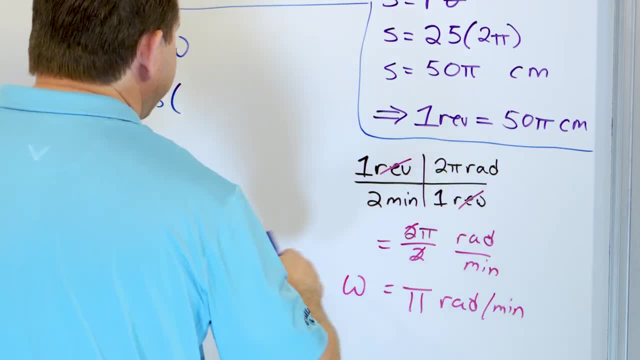 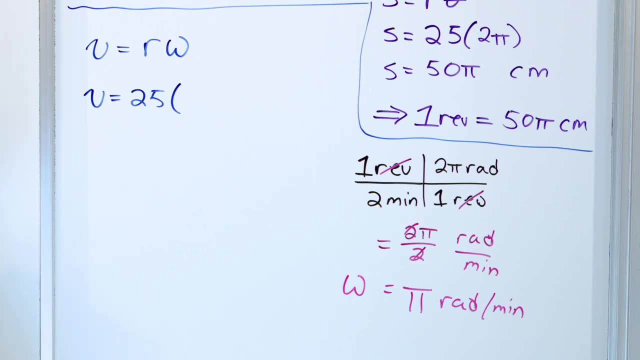 So, if you now know omega, which is radians per minute, and you know the radius, which is in the same unit of time, which is, in this case, or in the same unit of distance that you want, in terms of centimeters, 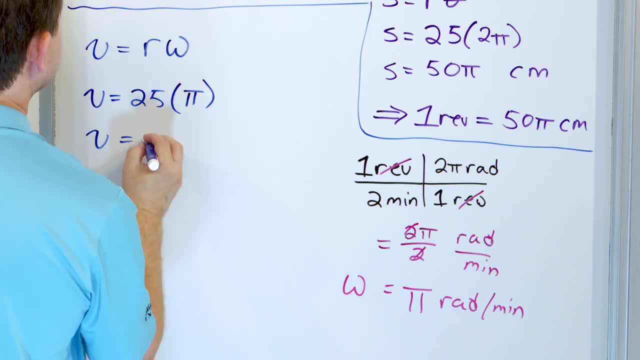 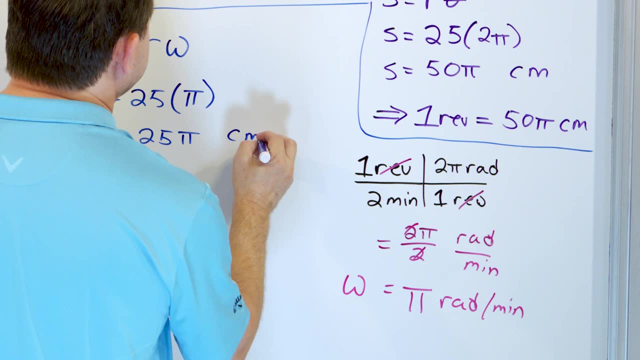 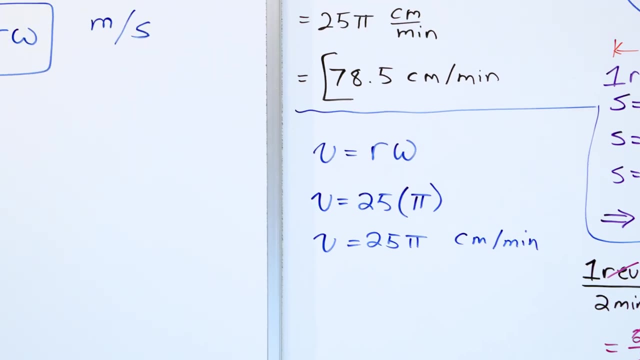 then we'll put pi in here, So 25 times pi, And then what you're going to get is, because you have centimeters here and you have minutes over there. it's centimeters per minute. So this is the way I think most books would probably want you to solve it in the beginning, right? 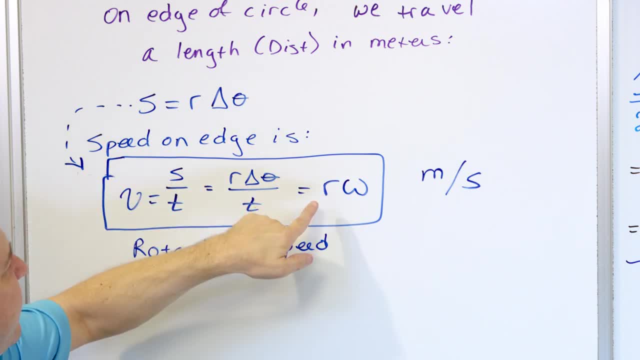 You would say I want the velocity on the edge of the circle. I can use any of these. I'm going to say it's the radius times, the angular speed. The radius is given to me. All I got to do is find the angular speed. 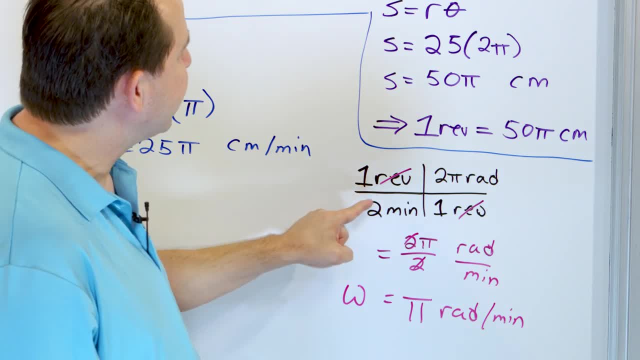 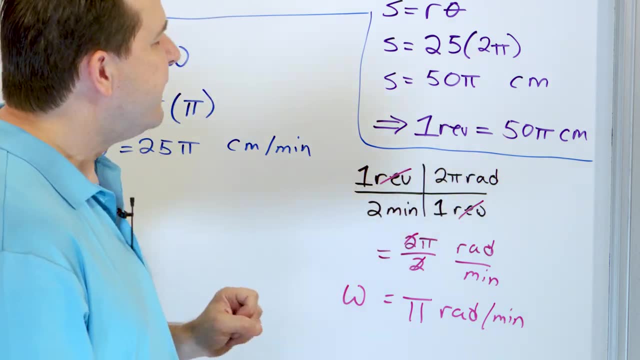 But I'm given the angular speed in a different unit: revolutions per minute. I convert it to radius. I convert it to radians per minute by getting rid of the revolutions, by knowing that one revolution is equal to two pi radians. Some sort of way, you have to know what these units are. 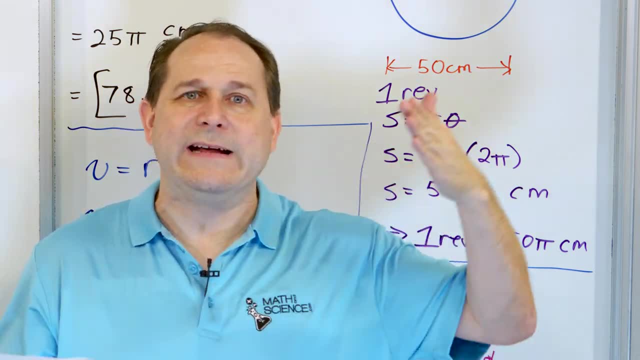 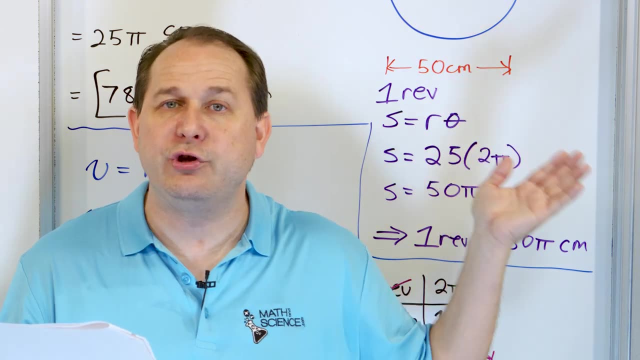 That's why I'm kind of going over it again and again. So you know, the angular speed is radians per, either radians per second or radians per minute, whatever you're working at. In this case, we wanted to keep it in minutes because the problem wanted the final units to be in terms of minutes. 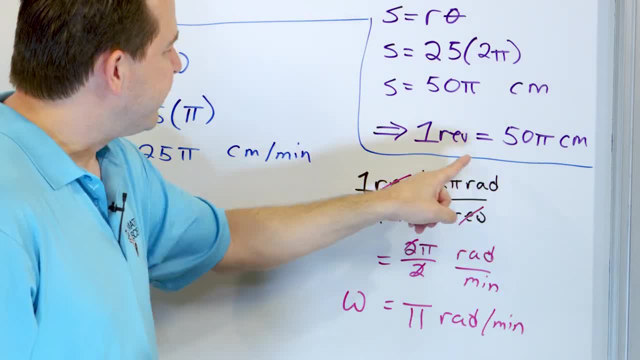 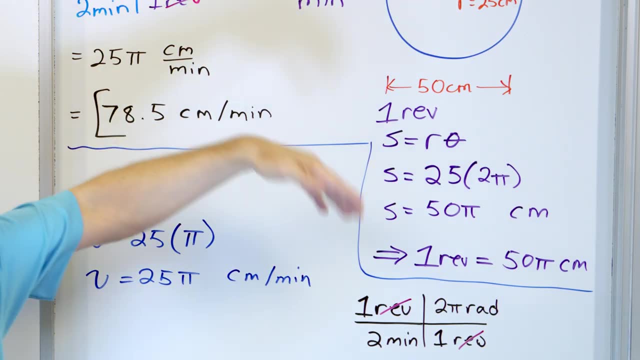 For that speed. they're centimeters per minute, So I convert it to radians per minute. This is omega, And then when you take omega times the radius, you get exactly the same answer as we got before, But where we really didn't even know what equation we were using. we're just trying to convert units to the correct place. 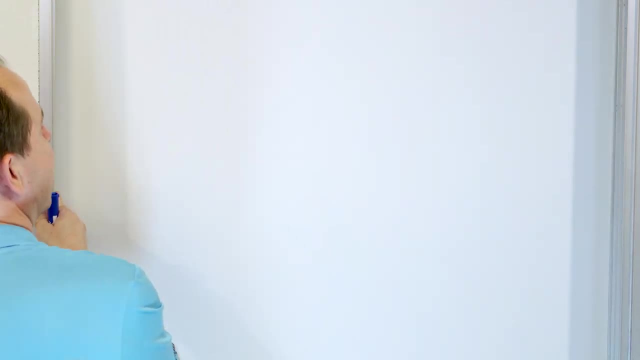 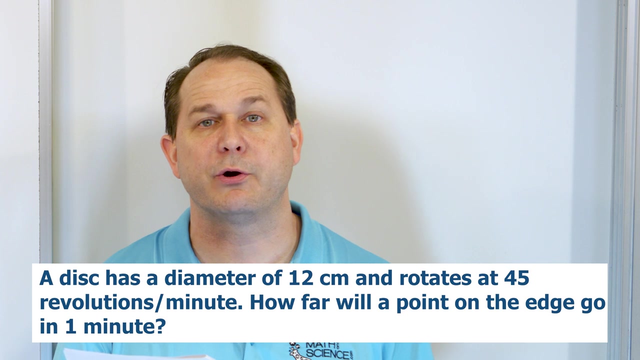 All right, Let's take a look at our last problem. A disk has a diameter of 12 centimeters and rotates at 45 revolutions per minute. How far will a point on the edge of the disk travel in one minute? So it's kind of asking you sort of the velocity. 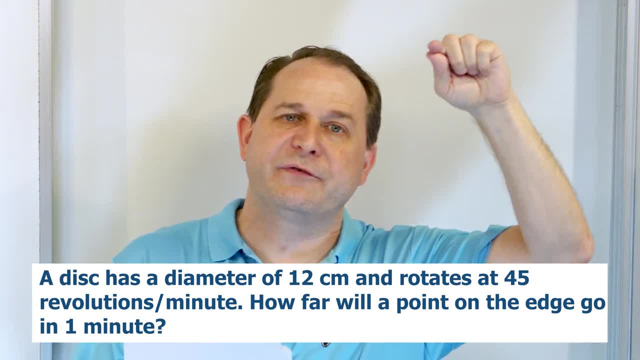 But really it's more asking you the distance. A point on the edge of the disk, A point on the edge of a circle travels in one minute. So what we want to do is take our baseline to be one minute and see what happens along the edge of the circle. 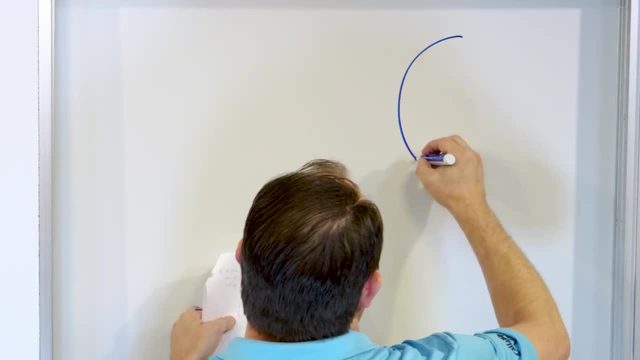 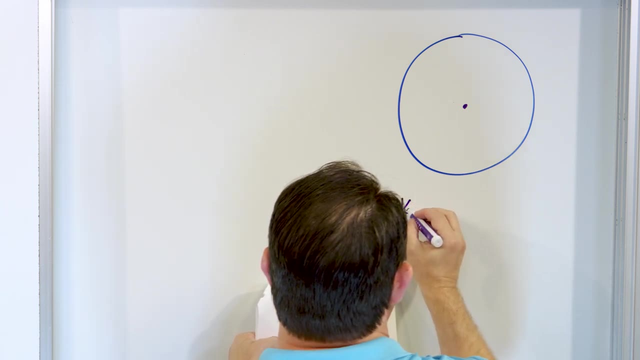 All right. So, as always, first we're going to draw a picture. So here is our circle like this, And let's draw what we know. So it says right here that the diameter is 12 centimeters. So that's the diameter. 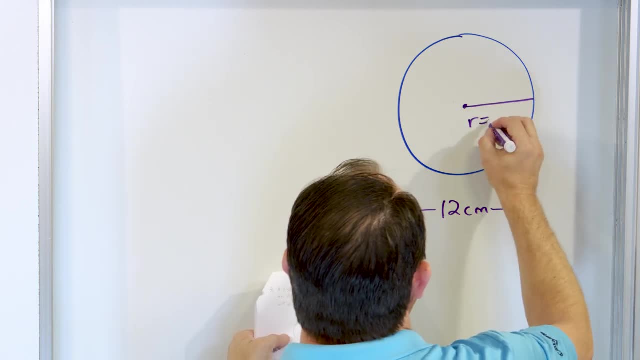 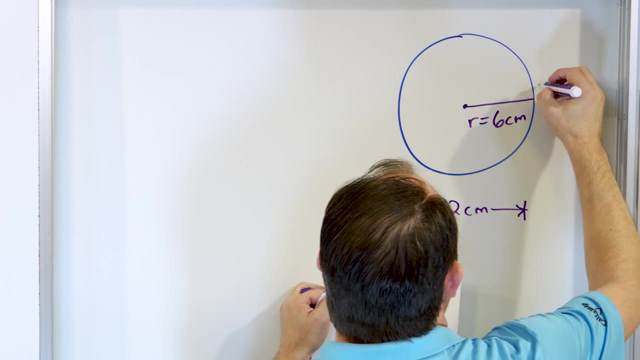 And so if this is the diameter, then the radius right here is six centimeters like this, All right. And then the other thing: it's telling us It's at 45 revolutions per minute. So I'll just draw a little error right here. 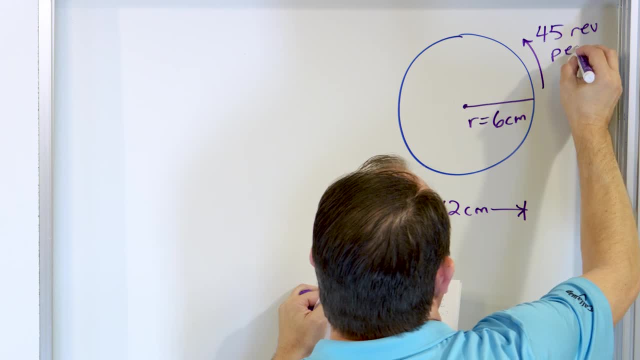 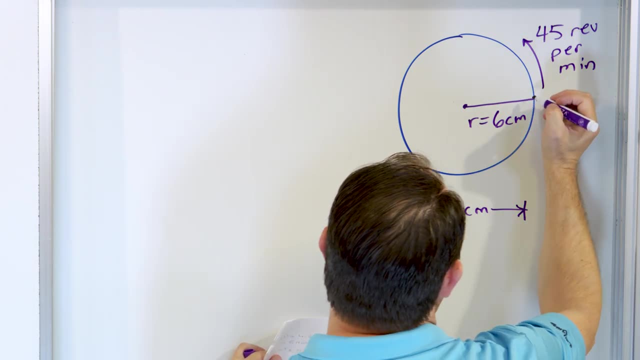 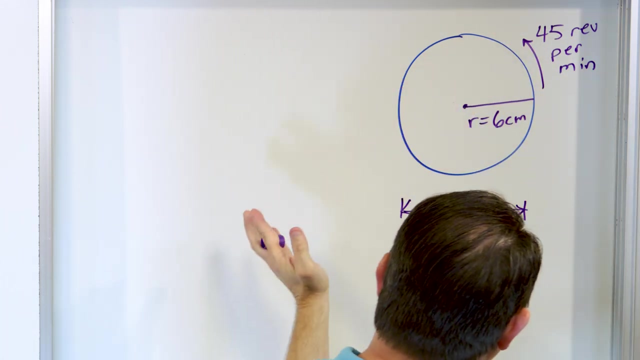 45 rev per minute. Rev per minute: OK, And then how far will a point travel in one minute? So basically, when we start here in one minute later and it moves, how far does it move? So what you're really asking is, how far along the arc does the thing travel in one minute? 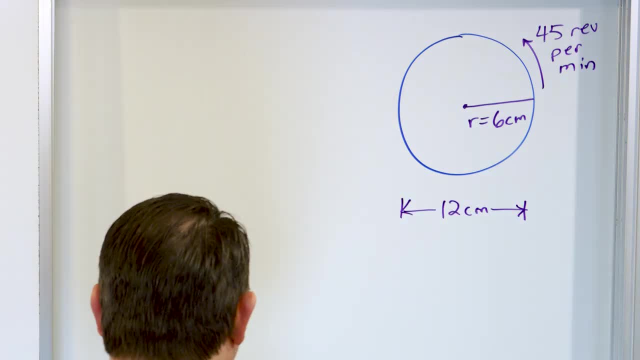 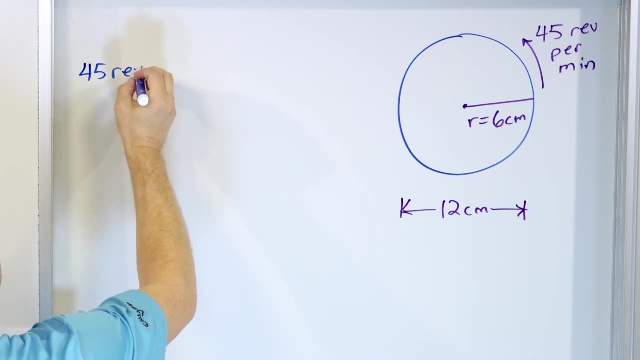 All right. So again, let's dispense and not even use the equations. Let's just write down what we know. All right, What we know is that we start off with 45 revolutions per minute. So we start off with 45 rev per minute. 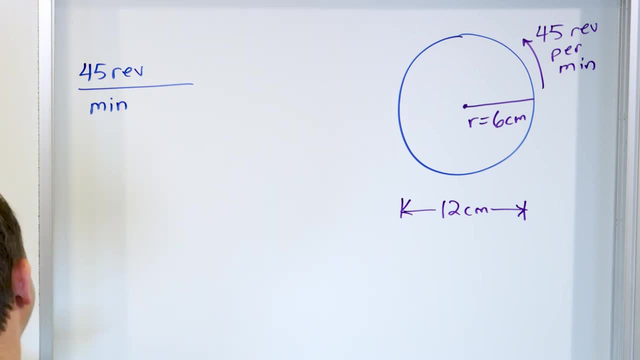 And that's a valid unit. 45 revolutions in one minute. Now this is a little bit silly, but the problem is asking us what happens after one minute. So we know it's 45 revolutions per minute. How many revolutions does the thing travel in one minute? 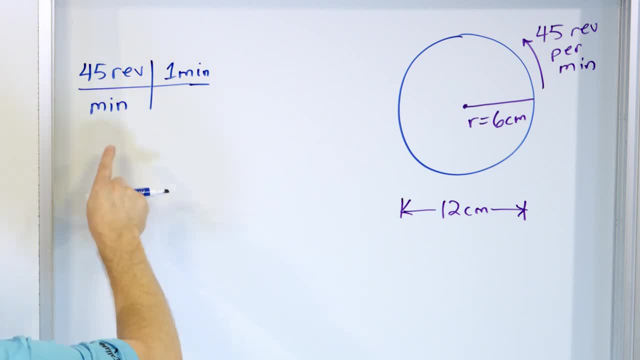 Well, we're just going to multiply by one. So if it's 45 RPM and you travel over a one-minute period, these cancel, And so it's 45 revolutions. 45 revolutions happen in one minute, All right, Now we want to figure out what is going on over one revolution. 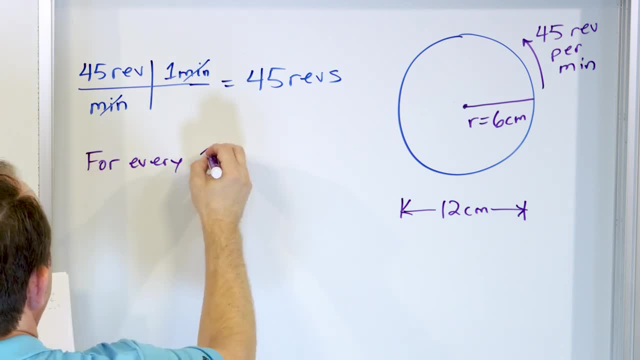 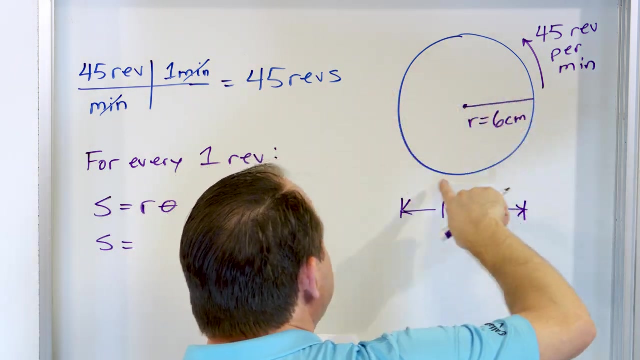 So for every one revolution that happens- because, notice, there's 45 revolutions that actually happen over a one-minute period- But for every one of these revolutions, we know s is r theta, And so the arc length that's traveling over a one-revolution period is just going to be 6.. 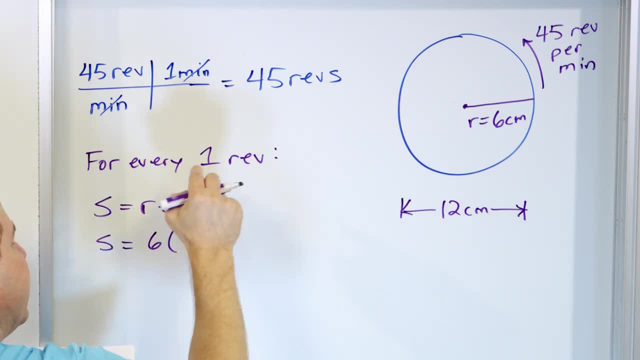 And what does that mean? And what is theta going to be? Over one revolution is going to be 2 pi radians, So what we get is 12 pi. And what's the unit of arc length? It's in centimeters, because this was in centimeters here. 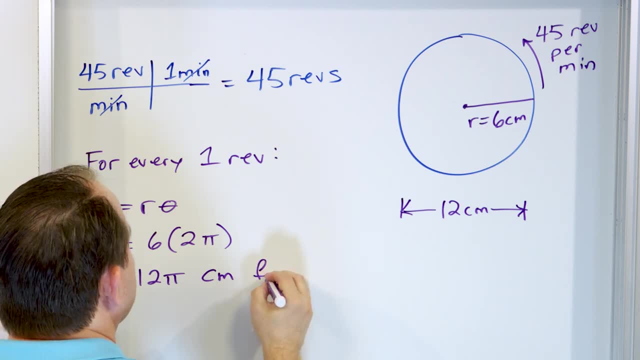 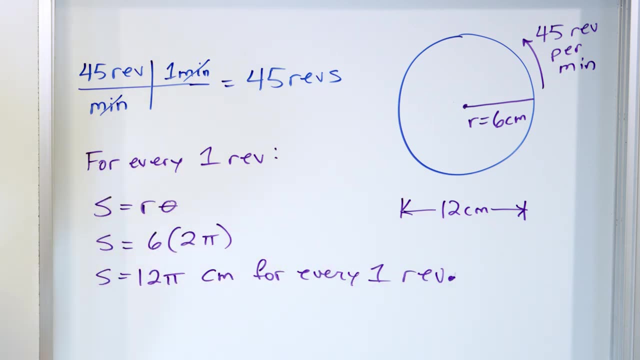 So centimeters for every one rev. So what have we figured out? What we figured out is this thing is rotating. Every single time it rotates, it goes all the way back to its starting point. Then, because of the radius and the angle that it rotates through all the way around, it travels this distance of centimeters every time it rotates. 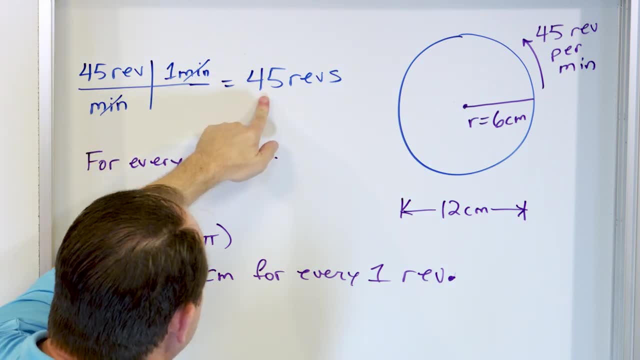 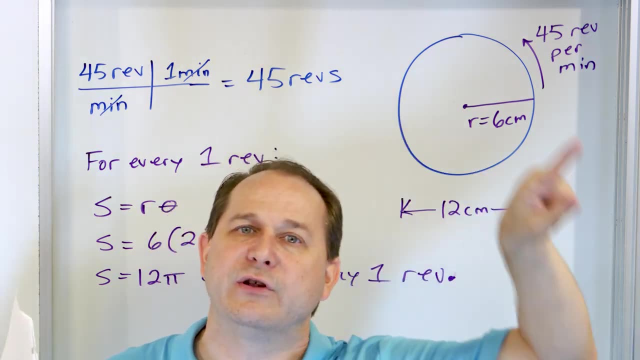 But then we figured out that in a one-minute period it actually rotates 45 times. So the question says: how far will a point on the edge of the circle travel in one minute? We know how many revolutions the thing happens in one minute. 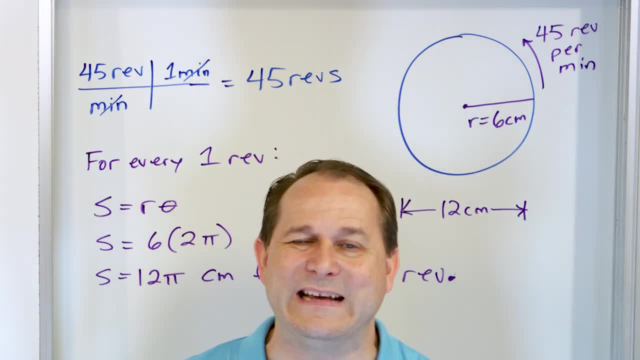 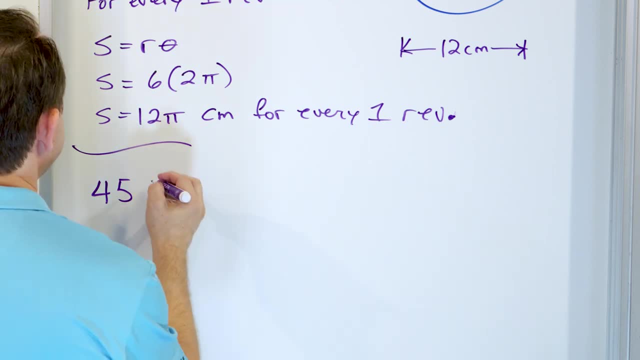 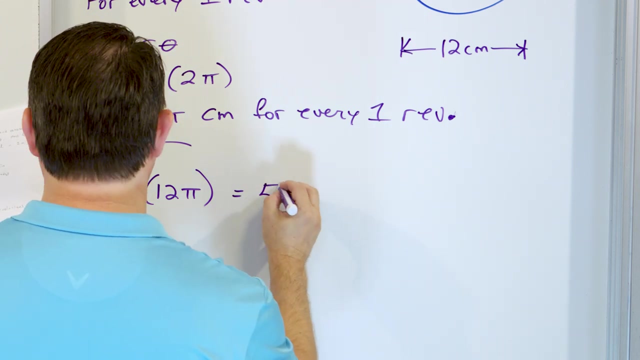 And we now know how far every one of those revolutions actually is. So we have to multiply those two numbers together, So 45 revolutions happen all together- And then multiply by 12 pi centimeters for every one of those revolutions, And so what you get is 540 pi, which is approximately equal to 1695.6,. 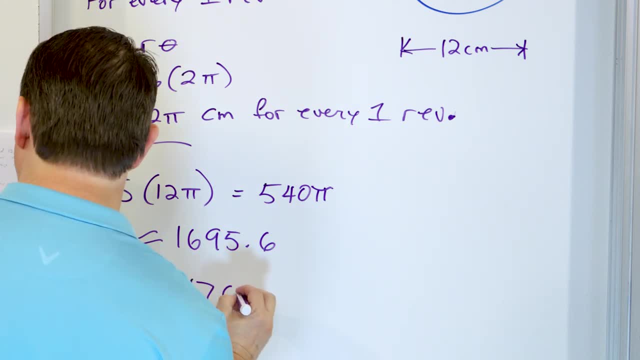 which is approximately equal to with rounding 1700.. And that's going to be in centimeters. Why? Because this is a unit of centimeters, The arc length is a unit of centimeters, and we do it 45 times. 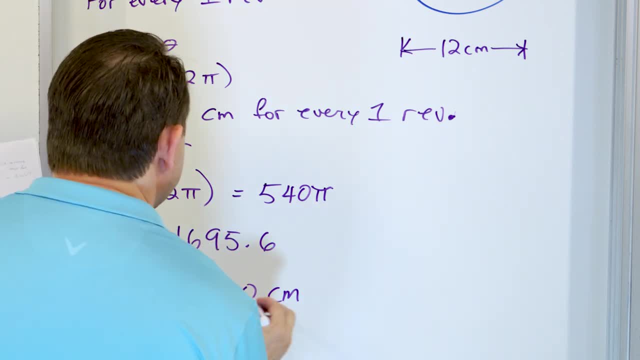 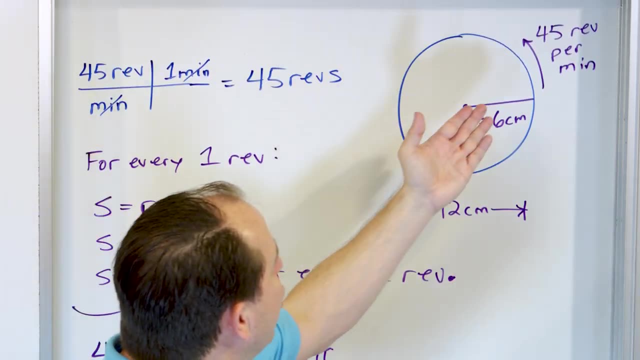 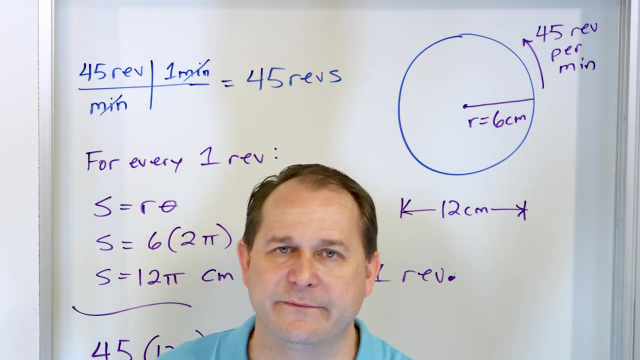 So the total unit is in centimeters Distance traveled in one minute. So it was kind of a two-part problem. The first part of the problem is we're told how fast this thing is rotating in terms of revolutions per minute. So we have to figure out over a one-minute period how many times does it rotate? 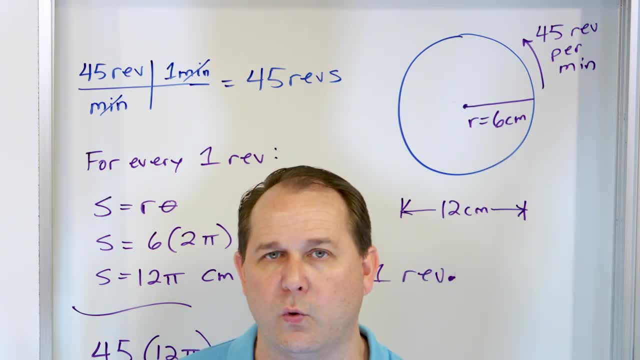 Well, it's kind of given to you in the problem. 45 times it rotates in one minute And then we just calculate how far around does it go every time it goes. Now I used arc length, but don't forget this is just the circumference of a circle, 2 pi r. 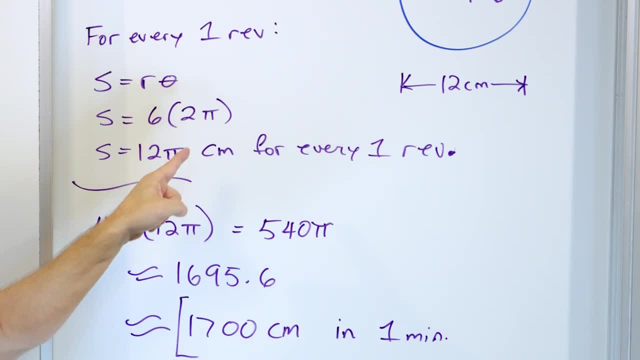 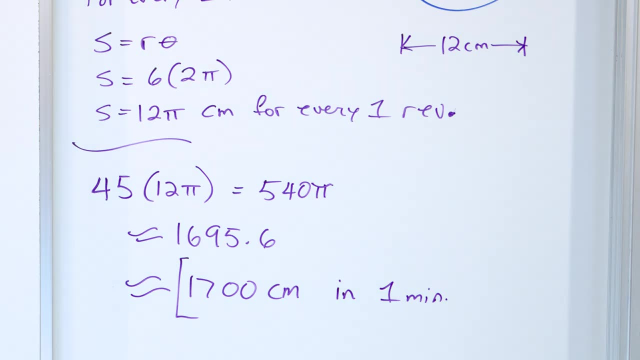 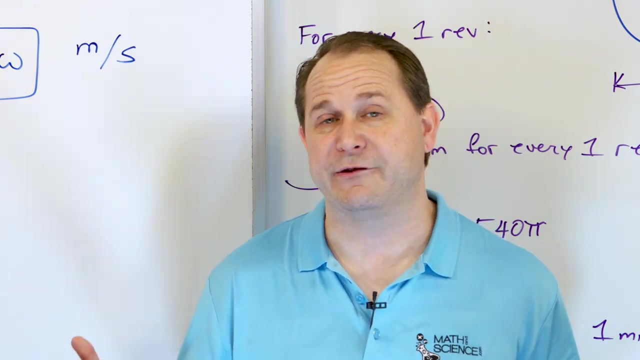 So this is the distance the thing travels over one revolution. So 45 rotations times. every revolution tells us how far this thing traveled altogether. Now I'm not going to lie to you. The first time I learned about angular speed and rotational speed, it was a little confusing. keeping it straight. 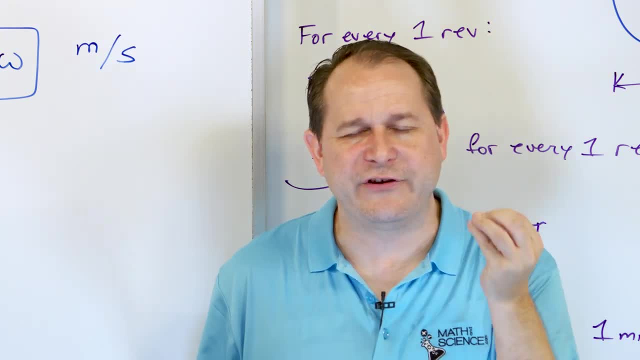 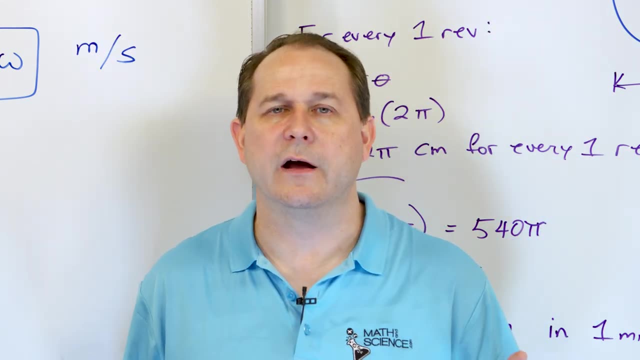 The only way you can get over that is by understanding the units and applying these to actual problems. So you have to get over this fear that you have initially of what is an angular speed. You have to get over that. You have to understand what radians are. 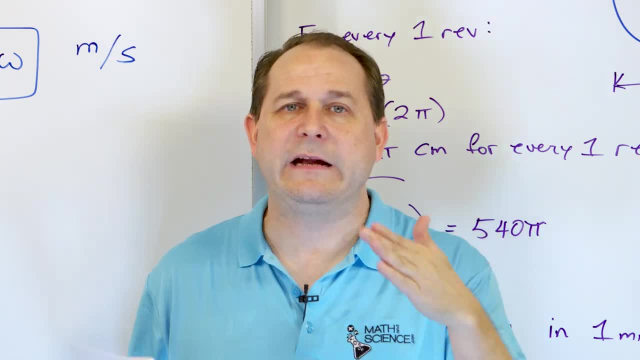 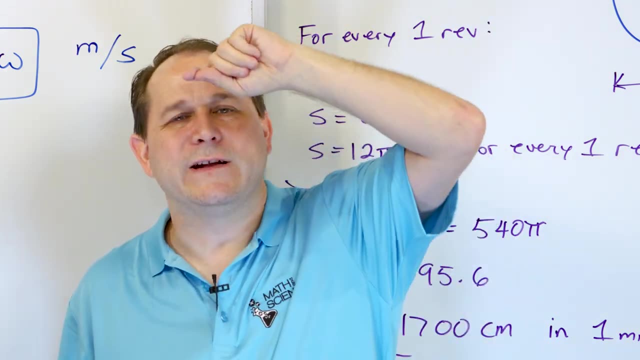 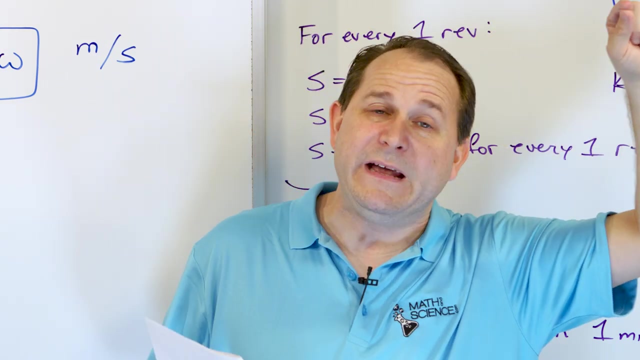 And realize that an angular speed is just radians per second or radians per minute or radians per hour, Some angle per unit time, But separate from that, along the edge of the circle a particle is traveling some linear distance over some time period. So it's going to travel some number of meters, which is along the curved arc length there.